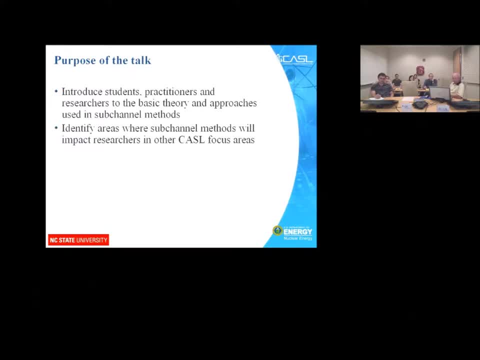 there. Cobra TF is the version that has been selected for use in CASL. It is not the only one out there, but it is one that has been selected for use in CASL. There's also VIPER, which is an EFRI version of the sub-channel code, which is used by many of the industry. 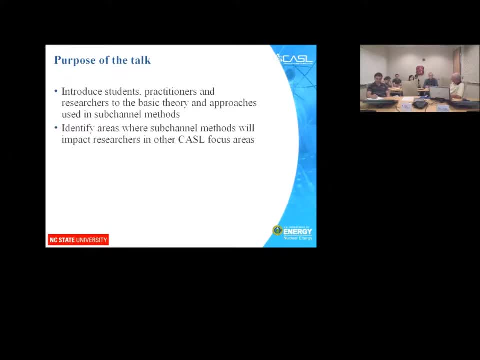 folks. Again, it was developed under EFRI sponsorship and that's the one I'm going to talk about today. I think that Westinghouse uses it, or a variant of VIPER. Again, these codes exist in various – a number of different versions. Many utilities or the vendors have adapted them for their 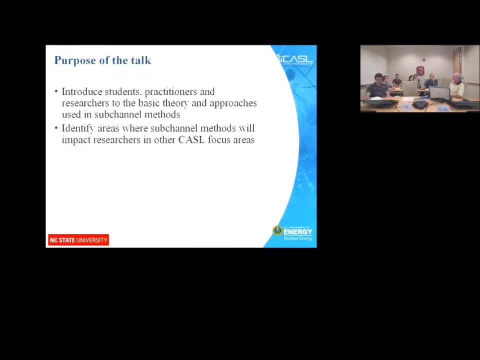 own use, put in proprietary correlations that are not available to others, But none of that matters for what we're going to talk about today. What we care about is: what are sub-channel methods? How are they used? What are the things that go into them? for example, One of the things that I would like 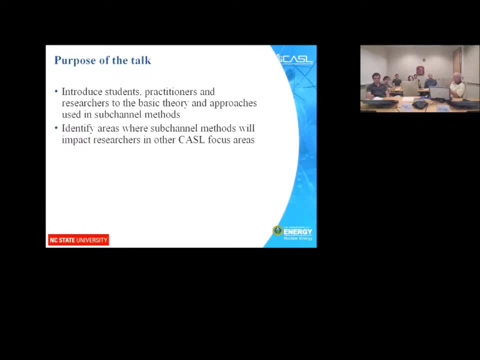 to do – and I'll try to do this over the course of the talk – is identify where these sub-channel methods are going to impact other researchers in the various CASL focus areas. For example, we have people at the UQ who are going to be trying to run Cobra or use. 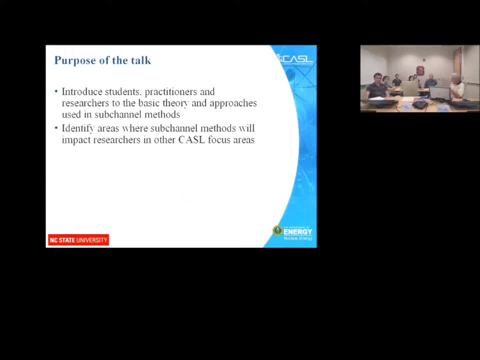 it: People in the transport methods, People in the chemistry methods. There are going to be various places that we're going to be looking at and trying to find solutions to, So we're going to have to look at. is there a way that we can use it? Are we going to? 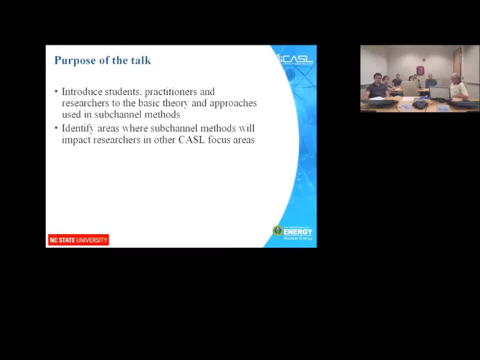 use it? Are we going to use it or not? Are we going to use it? Are we going to use it? Are we where people are going to have to interface with COBRA in one of the spurges? So they should at least have some idea of what's involved here. 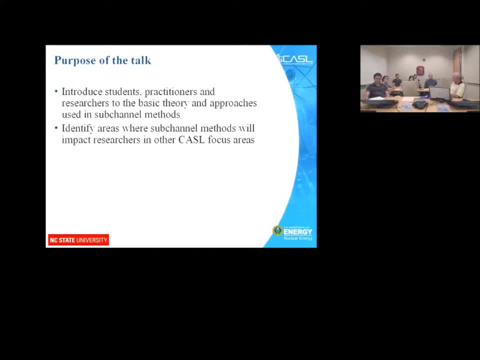 So this is going to be a talk. I'm going to try and develop the equation sets that are used to give people an idea of what the models look like and what the limitations are and where there are places where it will impact folks, I will again try. 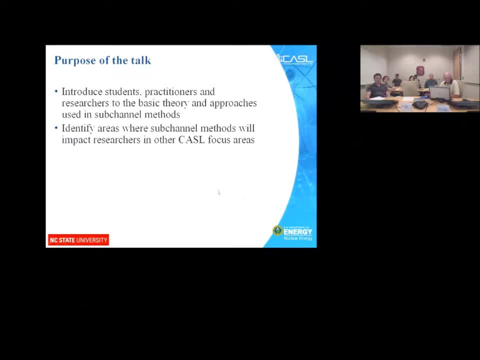 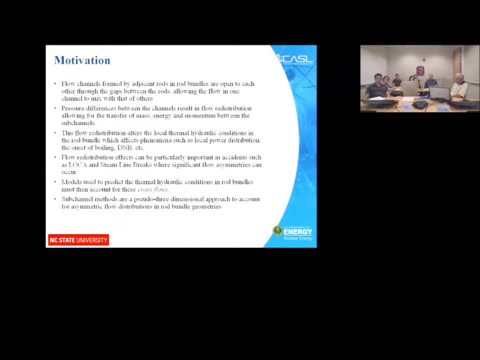 to point that out. This is a little busy, but the motivation for these four sub-channel methods are a number. One is- and I'm going to show you a picture of this in just a minute- the flow channels in rod bundles are actually between the rods themselves. 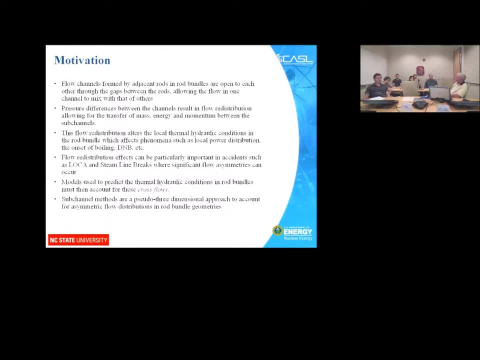 It's not around the rod, it's between the rods, And it doesn't matter whether you're talking about a rod bundle associated with a nuclear reactor, fuel bundle, Whether you're talking about an heat exchanger. you can use these codes to model all of that in some version of it. 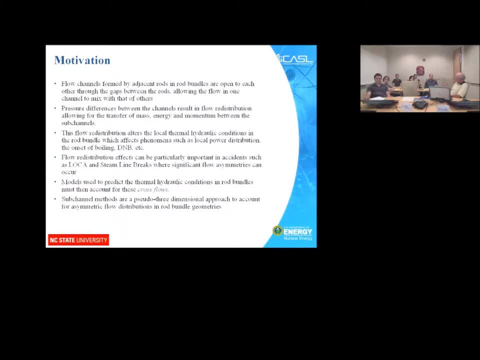 So the channels are formed between the rod bundles And, as a consequence of the channels being between these rods, there are gaps between the rods which allow flow from one sub-channel to move to the other and back and forth. So as a consequence of that, you have 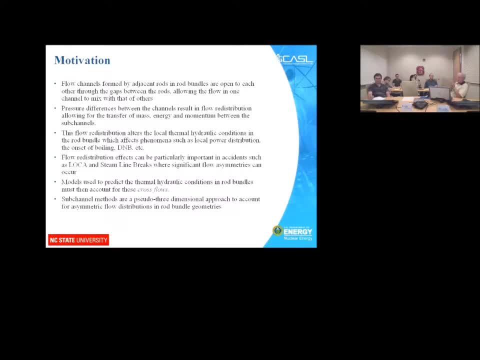 mixing between the sub-channels And these. if there are any differences in the rods that form these different channels- if there's any difference at all- that will result in pressure differences at an axial location at any point And those pressure differences will result in fluid moving from one sub-channel to the next. 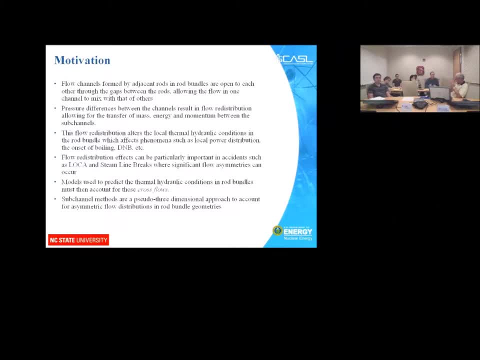 Now, when it does that, it's going to carry mass, It's going to carry energy, It's going to carry momentum And, as a consequence of that, the distribution, say, of energy in the channel is going to be a function of how much mixing occurs from one sub channel. 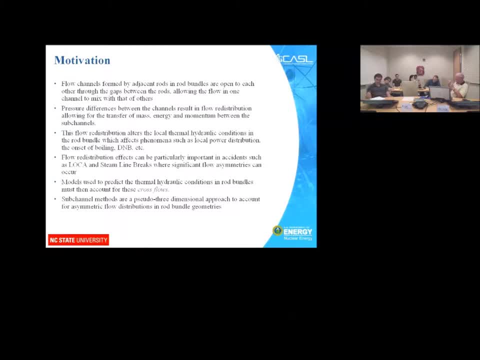 to the next. So if you have a local flow obstruction, for example in a channel, it will force fluid to move from that channel to another channel. If you have different heating rates in one channel relative to another, then the difference in the heating rates just different power. 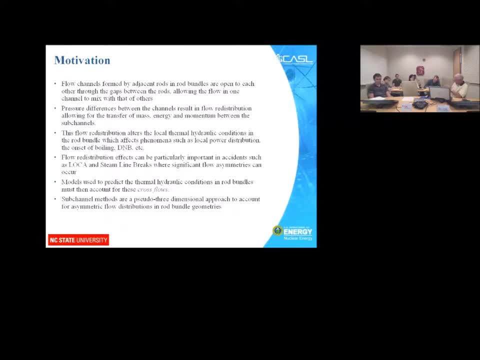 distributions in the rods themselves will result in different density distributions, different velocity distributions and, as a consequence, you will get fluid moving from one sub channel to the next sub channel, And I will use channel and sub channel interchangeably. A sub channel is simply that flow channel that exists between, that's surrounded by 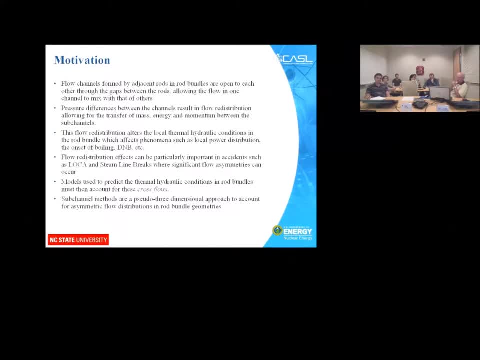 rods, And again, I'm going to show you a picture of this in just a moment. So again, if you have this flow redistribution fluid moving from one sub channel to another, then what that does is it alters the local, It alters the local thermohydraulic conditions, It changes the density, for example, Density. 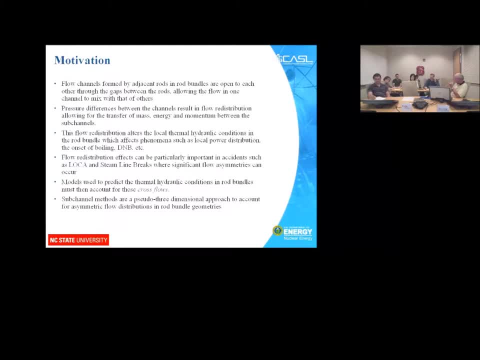 is important for people who are doing neutronics calculations because it affects the moderation that you have. If you have boiling, then that produces void and that void distribution also changes the neutron moderation, It changes reactivity, It changes the radiation transport calculations that you do. 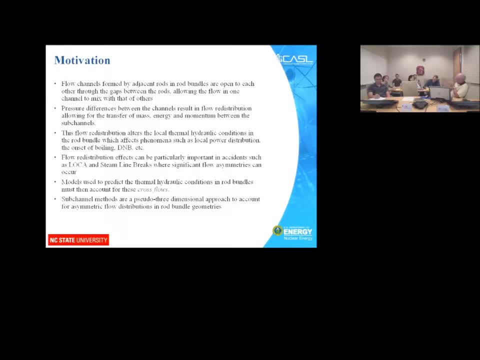 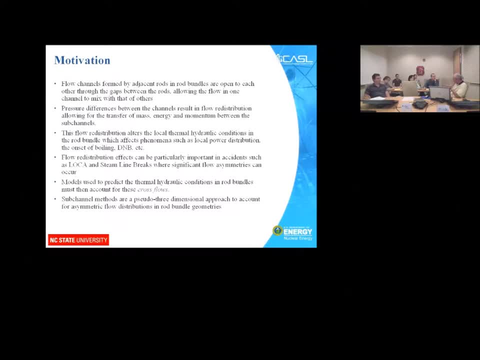 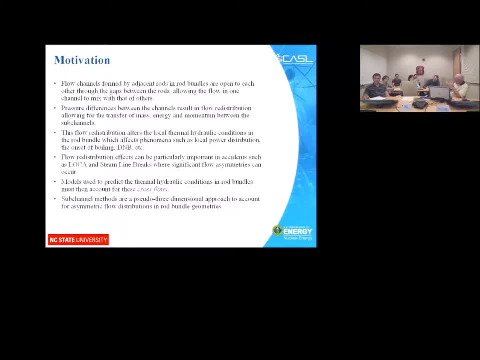 for nuclear boiling or other critical heat flux. The local fluid parameters directly impact where and if that occurs. While not necessarily at this point within the CASEL project, at some point they're interested in looking at some accident situations such as loss of coolant, accidents, LOCA or steam. 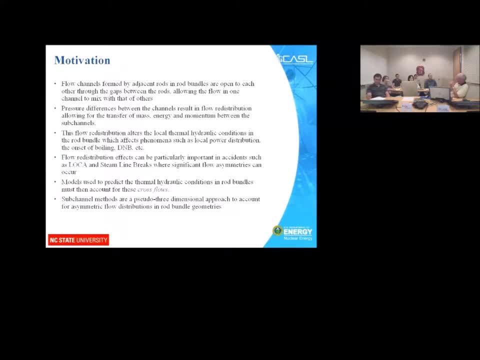 line breaks. In these cases you can have very large flow asymmetries, meaning that the fluid is moving from one part of the core maybe to another part of the core as a consequence of a pipe break. You have a large asymmetry in the pressure distribution radially across the core and 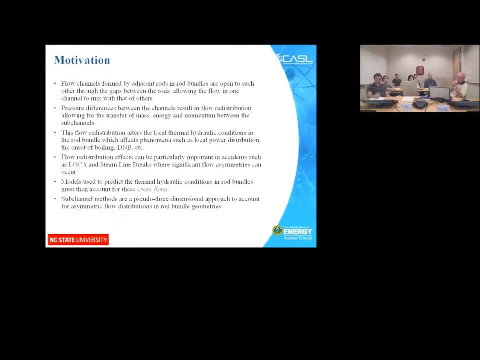 that will give you large flow mismatches. If we're going to try to calculate these kinds of phenomena, then we're going to have to be able to predict what these cross flows are: The flow transfer from one subchannel to another, The flow from one subchannel to another subchannel through the spacing between the rods. 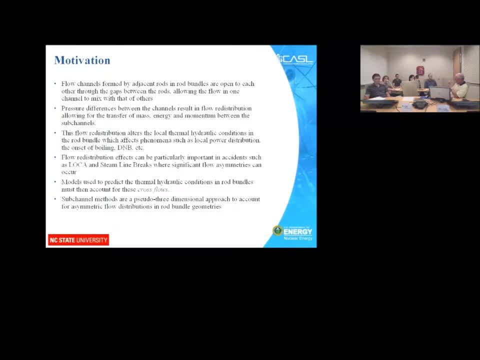 The subchannel methods are restricted to rod-bubble geometries. They are a pseudo-three-dimensional approach- and I'll show you what I mean by that as we go through this, but they are restricted to rod-bubble geometries. This is not a CFD calculation in its strictest sense, because you cannot use it to predict. 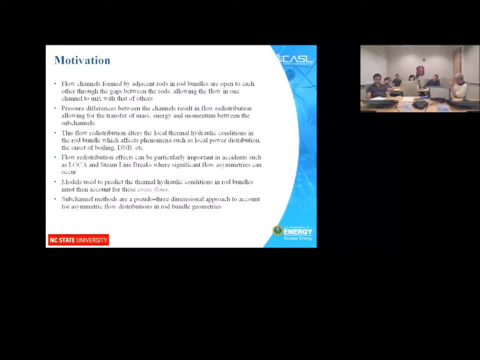 say three-dimensional flows in an open volume. It will not work. for that The methods, the models are derived, particularly for rod-bubble geometries. So again, if you've got some large open space, you really cannot predict three-dimensional. 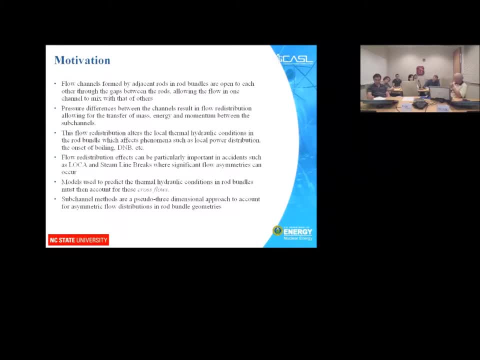 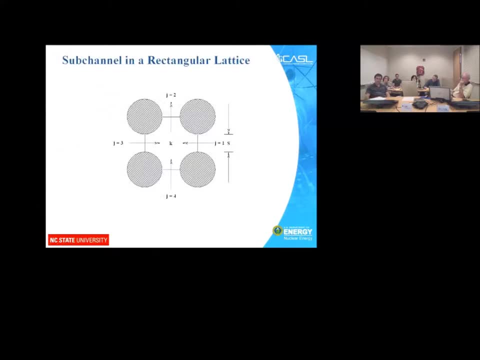 flow patterns in there. using these kinds of approaches It will not work. So I have illustrated here a subchannel in a rectangular lattice, and I'm going tothe discussion that we'll have today is for a rectangular lattice, even though there's nothing in the development of these. 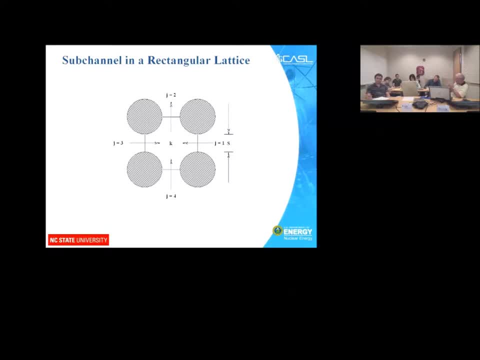 equations or applicability of them. that requires it to be a rectangular lattice. The equations are identical whether you're talking about a rectangular lattice, a triangular lattice or any other combination. All you have to do is be able to describe the interconnection of one subchannel to the. 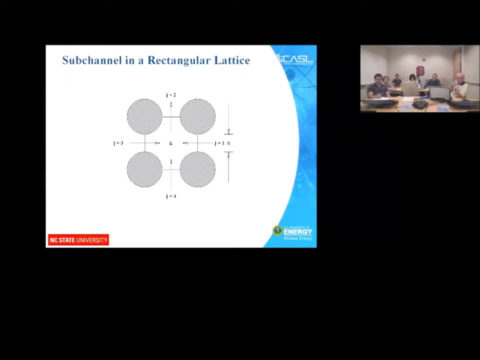 other, And so here I have indicated the subchannel which is indicated by K, And it's a subchannel. It's a subchannel And it is connected to four nearest neighbors. So I've numbered those J equal 1 to 4.. 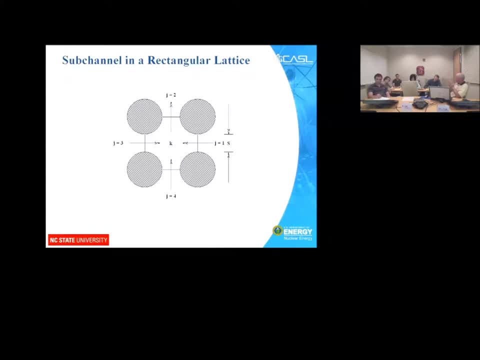 Obviously, if I have many subchannels then there are going to be many connections, But in general any one subchannel is connected to its nearest neighbors. So for example, in a triangular lattice it would be connected to its three nearest neighbors. 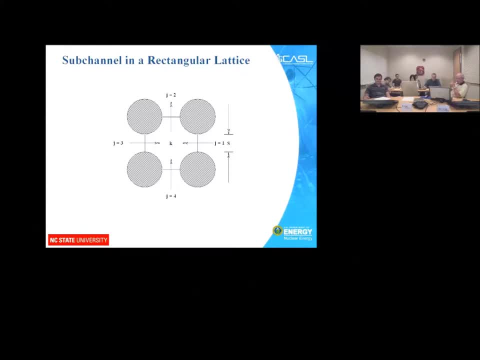 And in a rectangular lattice it's four nearest neighbors. All right, So that's one subchannel connected to its nearest neighbors And then each of the adjacent subchannels are connected to their nearest neighbors And you can enclose. For example, here I have shown just a subchannel that is open on all four sides. 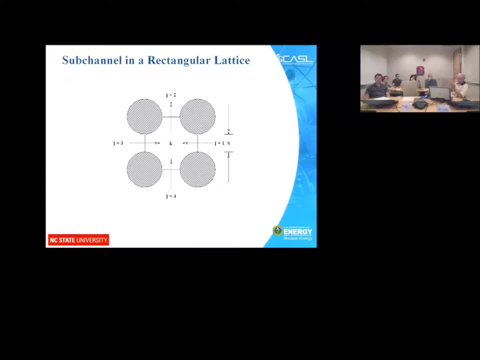 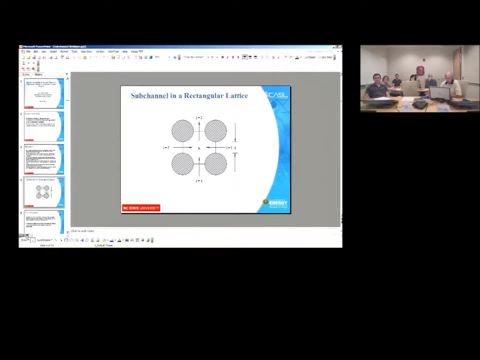 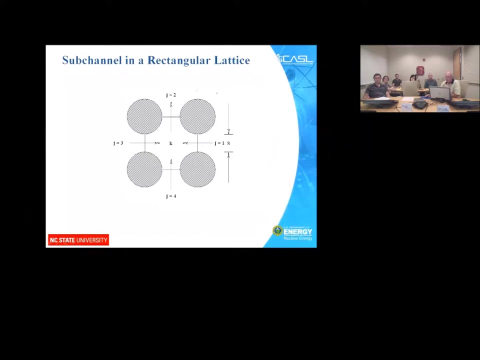 If I had a canned geometry, such as you might find in a boiling water reactor, then there may be – excuse me, Sorry, Sorry. Then if I've got a canned lattice, for example, then there may be a wall that would be here. 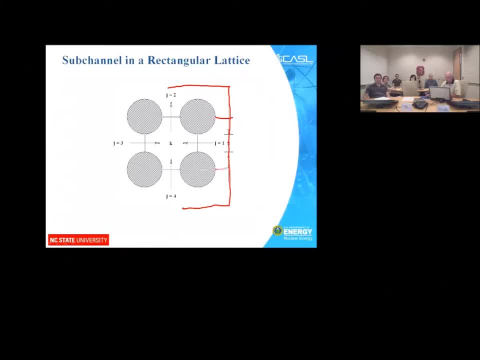 And then the subchannel would be, for example, that area right there. That would be a different side. So you are – the fact that I have indicated this as simply as with these four rods does not restrict it. Okay, You can have again a subchannel which is – okay, 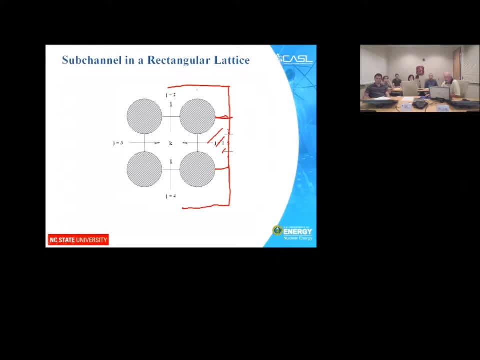 Okay, All right, So you would have a subchannel of this type and then you would have a corner subchannel again. This would be a separate subchannel type there also. So those are all a lattice. And again, when you set up the geometry you specify what the connections are, what subchannel. 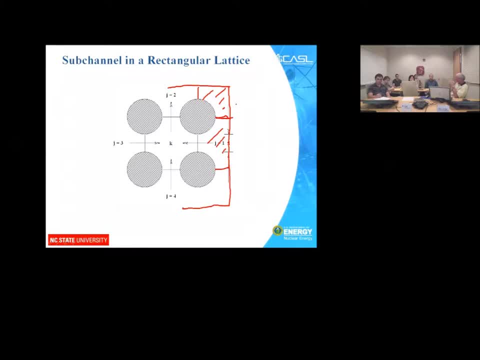 is connected to what other subchannels That connection geometry is set up and whether or not it is closed in or not, as I have indicated here. So those kinds of geometries can be modeled if you would like. Okay, So again this – so while I am going to be describing the development of the equations, 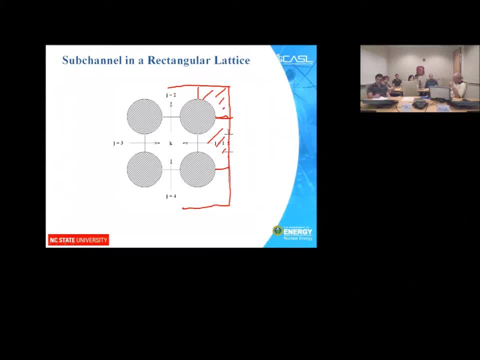 based on this generic sort of rectangular lattice. the equations are applicable to all of these other types as well. Now, when we talk about cross flows, we are going to be describing two – there are two unique types that are described or that are happening. 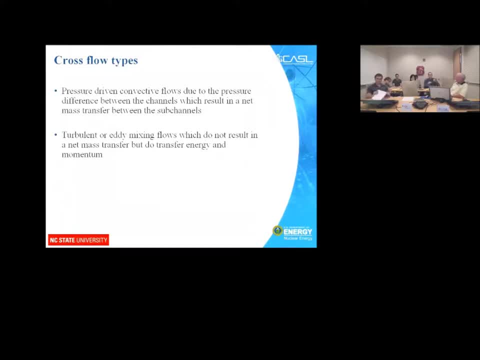 Okay, Or that are handled in these codes. One is the pressure-driven convective flows – okay – the pressure-driven convective flows that are the consequence of a pressure difference existing between two subchannels at any axial location. So if we have, for example, two subchannels that are immediately connected to each other. 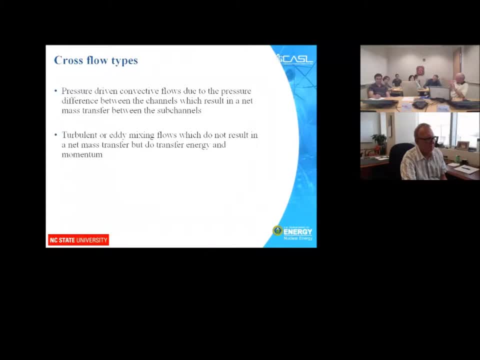 if there is a pressure difference – a lateral pressure difference – if there is a lateral pressure difference between those subchannels, at that point then you will get a pressure-driven convective flow as a consequence of that pressure difference. Okay, That one is relatively easy to describe. 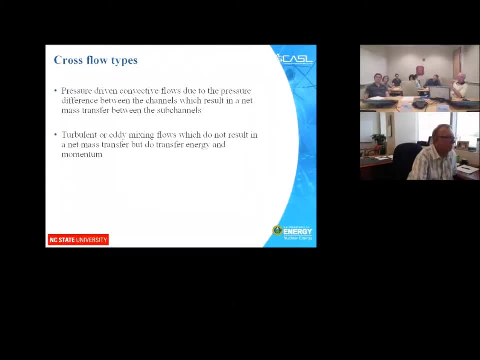 And we will talk about how we do that here in a moment- And these pressure-driven convective flows result in a net mass transfer between the subchannels. Okay, And that is the key difference between the two different types. So if I have a pressure-driven convective flow, then I have a pressure-driven convective. 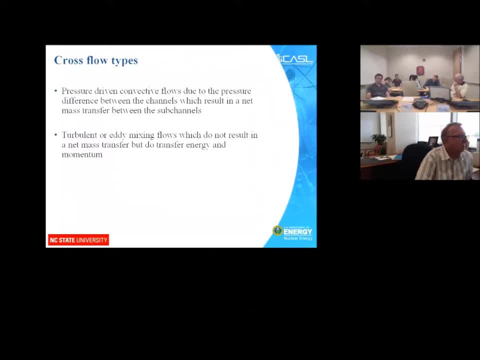 flow. If I have a pressure-driven cross flow between two subchannels, then there will be a mass – there will be net mass transfer between the – between those two subchannels, Okay, And that mass transfer will carry energy and momentum with it, but there will be also a 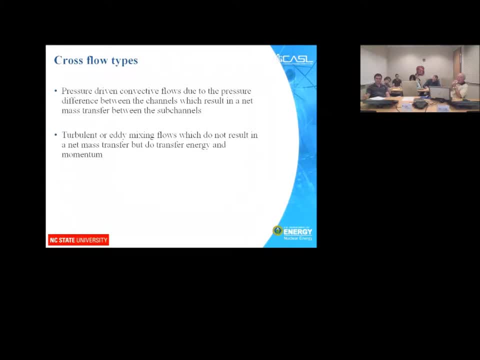 net mass transfer between those two channels. There is a separate type of cross flow, which is included in these models, which is called a turbulent or eddy mixing flow, Which does not – Okay, There is no transfer mass, There is no net mass transfer as a consequence of this flow. 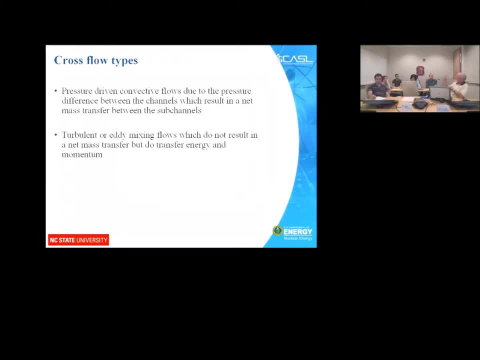 So the way that I like to describe it is think of a little whirlpool sitting between channels, so that whatever flows in immediately turns around and flows back out again. But as a consequence of that flow in and flow out, there is a transfer of energy and momentum. 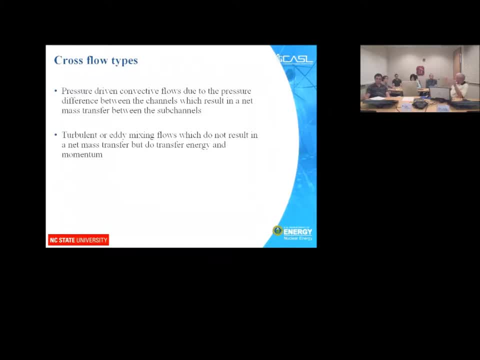 So even if there were no pressure differential between two channels so that you didn't get any pressure-driven flow, if they had different enthalpies or temperatures- if you want to think about it that way- then these turbulent mixing flows would end up trying to equalize the 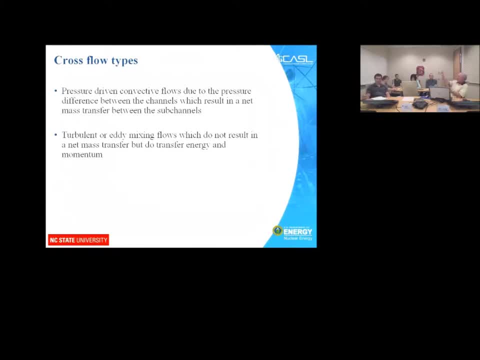 enthalpy distributions across all of the channels. You would not have a hot channel on one side and a cold channel on the other, and they would remain that way. Because of this turbulent mixing, they would tend to equilibrate between them. 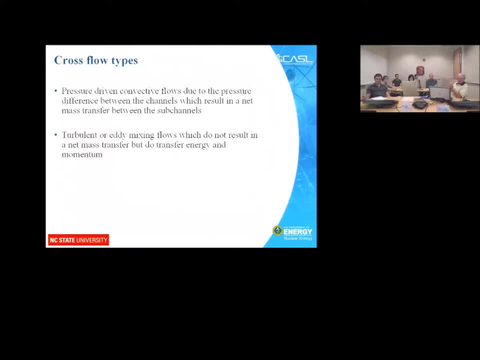 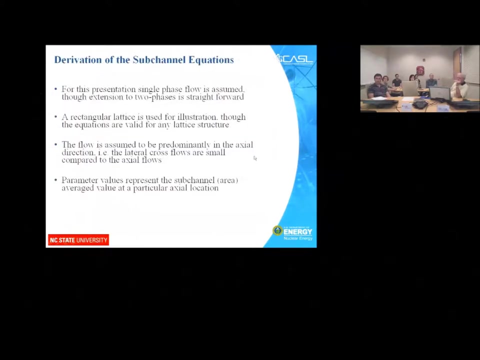 So this is a second type of cross flow, So the equations contain terms in them which represent the flow. Okay, Okay, So what I'm going to do is walk you through the derivation of the sub-channel equations. If you are trying to work with sub-channel codes and you look in the manuals, they're 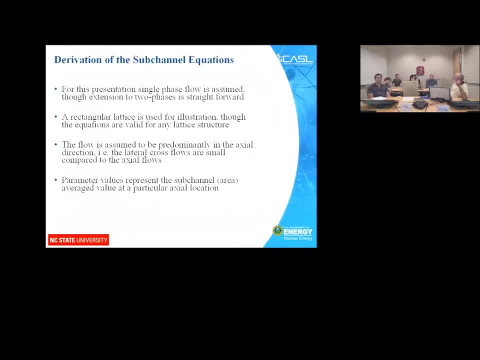 going to give you these equations, And so you might as well know where they come from and have some idea of where they're from, And it will also, as a consequence of this, I will point out, as we're going through this derivation, what terms might be of particular interest to different folks. 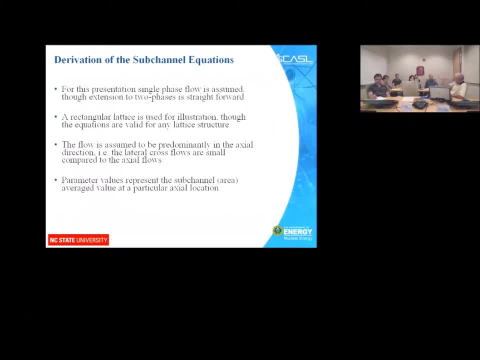 For example, if there's a correlation in here you might want to know: okay, this is a correlated parameter, something that the UQ people may want to fiddle with, okay, or look at, alter it or modify it. 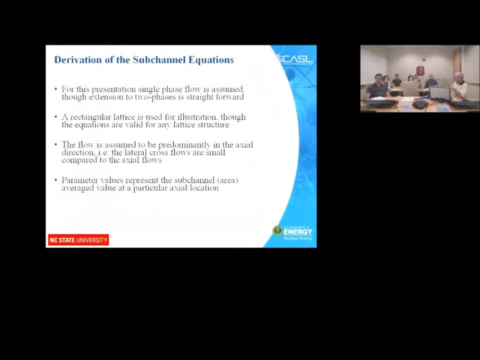 Okay, So I'm going to assume again to keep, so we can keep the algebra down and keep all the discussion running. Okay, It's going to be rather simple. I'm going to use single-phase flow for this discussion. The extension to two phases is relatively straightforward. 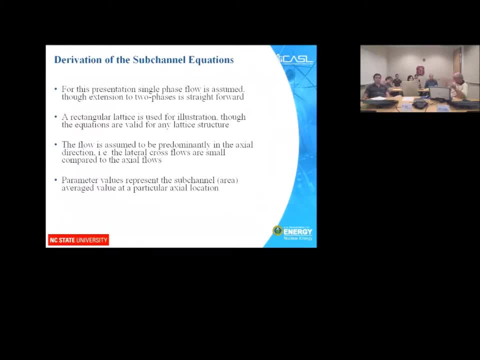 Okay, There's no. you just apply it to two different phases And this is not a, this is not a discussion of two-phase flow models. That's a whole different, whole different seminar. But if you have, if you have looked at two-phase flow at all- and I think we have people in- 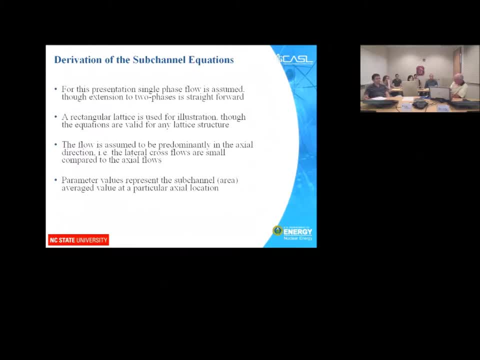 the seminar series who are going to give two-phase flow. If you're going to give a two-phase flow presentation, then the application of those to the sub-channel approach is straightforward. Okay, It follows the exact same approach to what I'm going to do here. 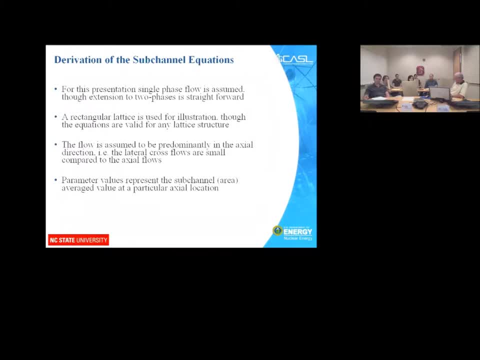 So I'm going to just do this for single-phase flow. If we can't understand what's going on with single-phase, there's no way in the world we're going to get it for two-phase. I'm going to use the rectangular lattice that I illustrated below for illustration, though. 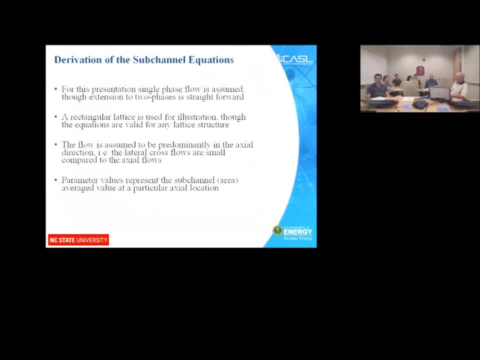 again, the equations that we're going to develop are going to be as you'll see. they will have nothing in it which is lattice dependent, So it will have things in it, for example, the distance between the sub-channels. Okay, 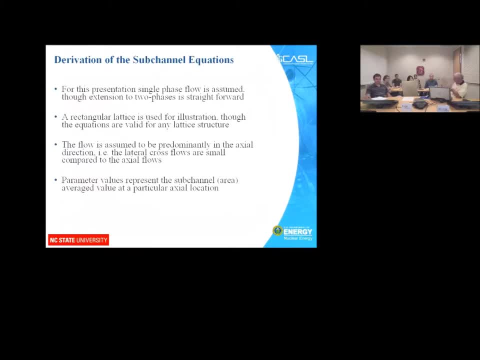 It will have any cross-sectional areas, gap spacings that you can use to describe any lattice structure that you want. So all you have to do is say this sub-channel is connected to this sub-channel in the input And this sub-channel will have certain characteristics, an area, for example, 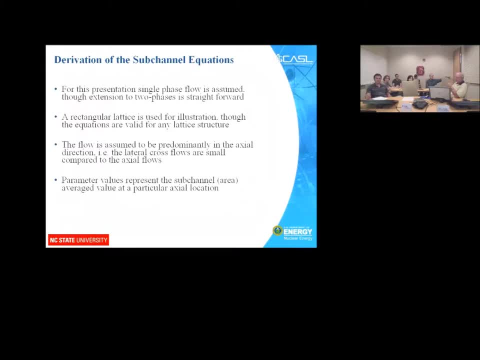 One of the primary assumptions is that the sub-channel is connected to the input. Okay, So this sub-channel is connected to the input, This sub-channel is connected to the input and this sub-channel is connected to the input. So we have to make sure that we're getting the right direction for the process. 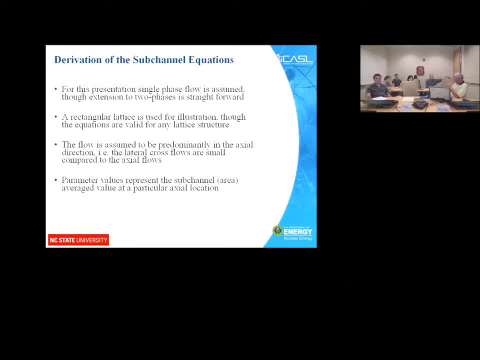 And this is one of the main assumptions in the sub-channel equation- is that the flow is predominantly in the axial direction. So that is an inherent assumption in development of these equations, that by axial it doesn't mean necessarily vertical, but axial is the dominant flow direction along the parallel. 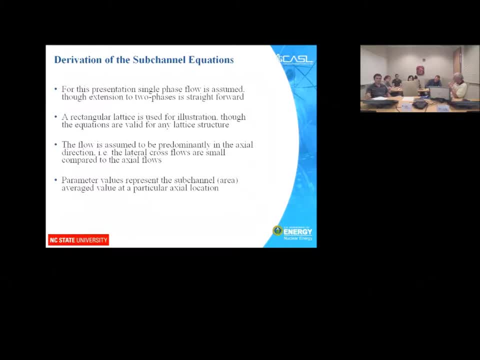 to the log bundles. Okay, So by axial flow, I'm going to mean flow parallel to the log bundles- is assumed to be the dominant flow in all of this And that the lateral cross-flows, Okay, are relatively small compared to those. 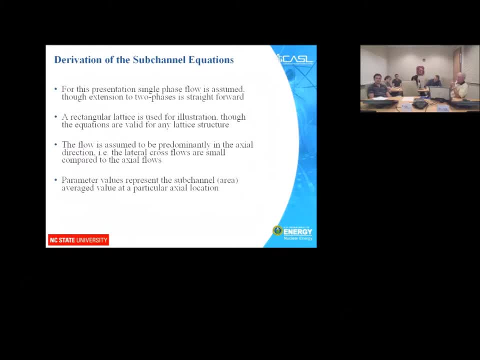 That is an assumption that you find inherent to all of these sub-channel type codes. Now, the other thing that is inherent in the assumptions are the parameter values that you predict, whether it's density, enthalpy, temperature, velocity. These are the sub-channel area average values. 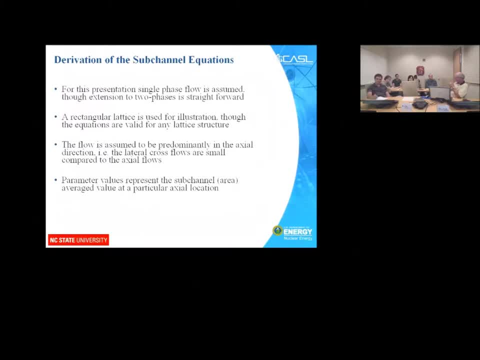 at that particular axial location. So if I predict a density at an axial point within a sub-channel, then that density represents the area average density over that sub-channel. If I predict a velocity in the axial direction for that sub-channel at that location, 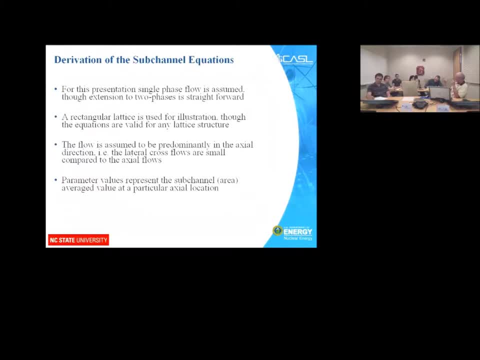 then that is the area average velocity for that sub-channel. Okay, So the parameter values again represent the sub-channel or area average value at a particular axial location, And that is in the radial direction. There is no finer meshing that can be done. 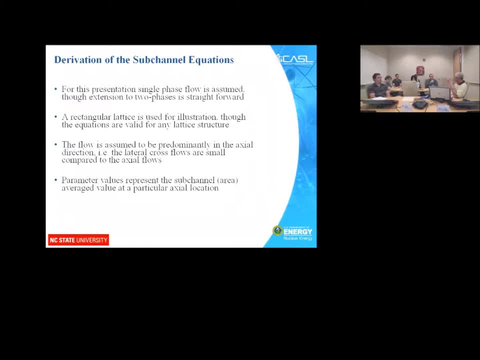 The mesh is the sub-channel That is the smallest in the lateral direction. Okay, You can choose whatever axial mesh generally you want to, but there is no fine mesh. There is no finer meshing in the lateral direction than on a sub-channel basis. 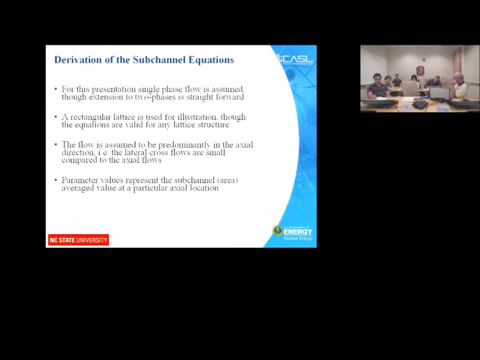 So you cannot go into these codes and subdivide the sub-channel, okay, and predict different parts, Okay, Okay. So most of the time, what you see when these code, when the equations are developed, or the 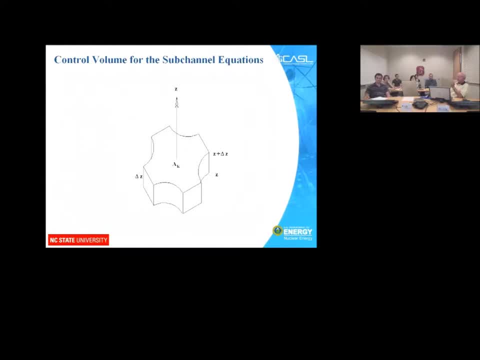 It is sort of a classic control volume approach to developing these equations, and that is the one that I am going to follow. 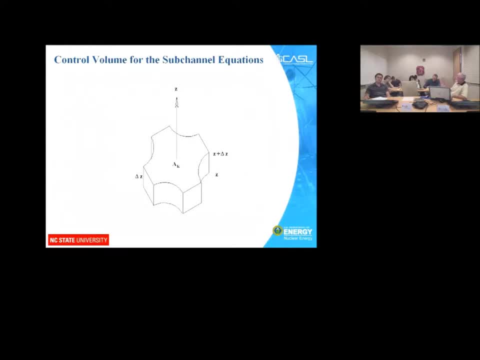 It is physically based, You can. There are much more rigorous ways to go about generating these area average equations. You end up ultimately with the same equations. It is just the definitions of what the average means is different, but they all look the same. 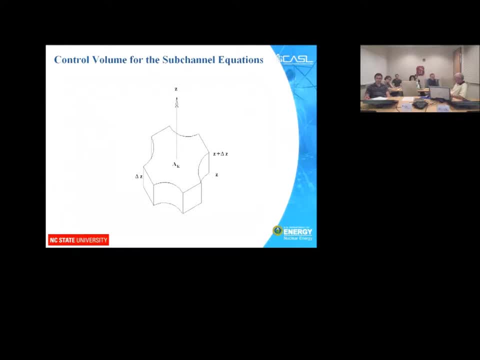 So the sub-channel- Again, this is for a rectangular sub-channel and the, the equations that will develop are based on a control volume of this form. so again here, if you look at this area right here, represents the contact of the. 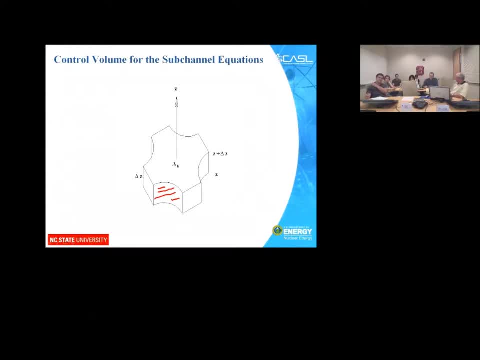 that's where the rod is in contact with the fluid. okay, the gas would be here. okay, but these surfaces at this point represent those are the lateral flow surfaces. okay, across the flats, if you will. okay, that's a lateral, again, a lateral flow surface. okay, across the flats, if you will. okay, that's a lateral, again, a lateral flow surface. 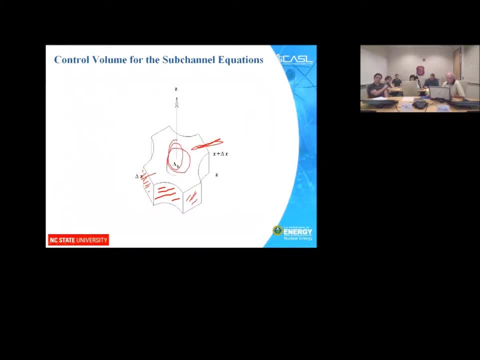 okay, across the flats, if you will okay, that's a lateral, again, a lateral flow surface. and then this big area here that is okay, across the flats, if you will okay, that's a lateral area here. that is okay, across the flats, if you will okay, that's a lateral area here. that is denoted by a sub K, that big area there is. 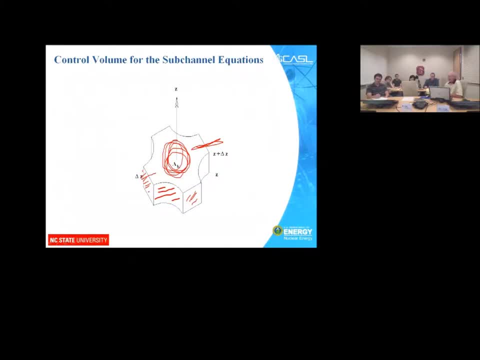 okay, that's a lateral area here. that is denoted by a sub K, that big area there is- okay, that's a lateral area here that is denoted by a sub K, that big area. there is the axial flow area and then I've denoted Z. 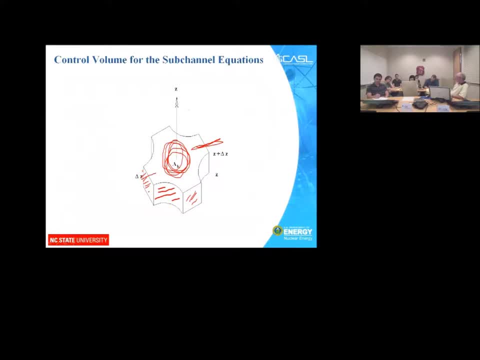 denoted by a sub K, that big area, there is the axial flow area. and then I've denoted Z, denoted by a sub K, that big area, there is the axial flow area. and then I've denoted Z here in the axial flow direction, even. the axial flow area, and then I've denoted Z here in the axial flow direction, even the axial flow area, and then I've denoted Z here in the axial flow direction, even though, for example, if the castle ever here in the axial flow direction, even though, for example, if the castle ever 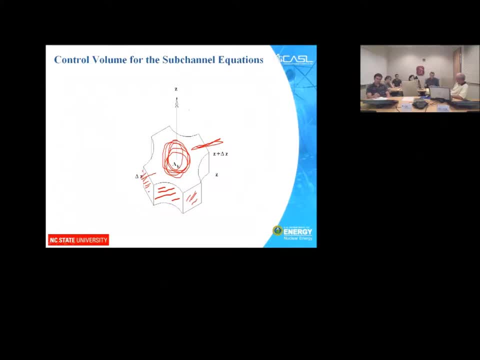 here in the axial flow direction, even though, for example, if the castle ever decided that it wanted to model, can do though. for example, if the castle ever decided that it wanted to model, can do though. for example, if the castle ever decided that it wanted to model, can do reactors where the bundles run horizontally. 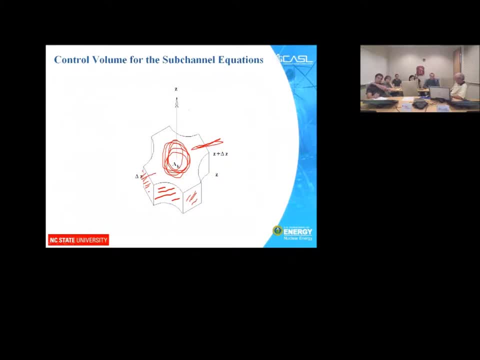 decided that it wanted to model can do reactors where the bundles run horizontally. decided that it wanted to model can do reactors where the bundles run horizontally. Z would be part in the horizontal reactors where the bundles run horizontally. Z would be part in the horizontal reactors where the bundles run horizontally. Z would be part in the horizontal direction, even though that's the axial flow. 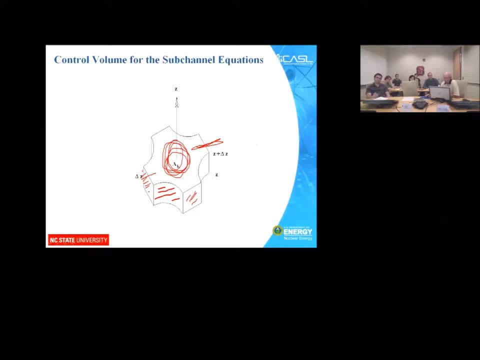 Z would be part in the horizontal direction, even though that's the axial flow. Z would be part in the horizontal direction, even though that's the axial flow direction. okay, and so again we'll walk direction. okay, and so again we'll walk direction. okay, and so again we'll walk through this. we'll do the easiest one. 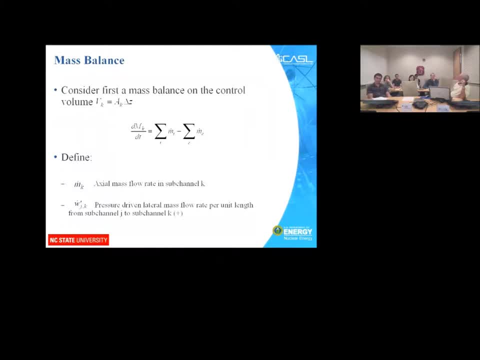 through this, we'll do the easiest one. through this, we'll do the easiest one first and again this. so I have to tone first and again this. so I have to tone first and again this. so I have to tone this for people who may not be engineers: 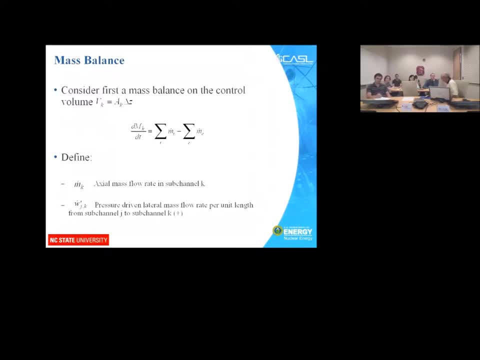 this for people who may not be engineers, this for people who may not be engineers. there may be wherever the back next, but there may be wherever the back next, but there may be wherever the back next. but certain things we can certainly talk. certain things we can certainly talk. 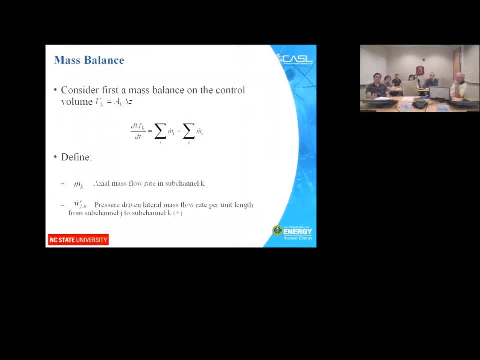 certain things. we can certainly talk about a simple mass balance, about a simple mass balance, about a simple mass balance, and the we're going to take it perform a and the we're going to take it perform a and the we're going to take it perform a mass balance. on this indicate here. 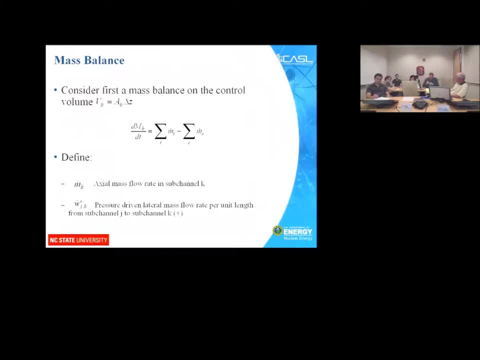 mass balance on this indicate here. mass balance on this. indicate here: denotes sub channel K. it does not denote: denotes sub channel K. it does not denote, denotes sub channel K. it does not denote an axial location. okay, so there would an axial location. okay, so there would an axial location. okay, so there would end up in multiple subscripts if you. 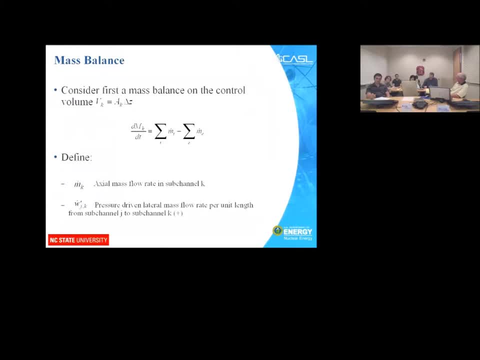 end up in multiple subscripts. if you end up in multiple subscripts, if you were to discretize one of these one, were to discretize one of these one, were to discretize one of these one would be sub channel K, maybe axial. would be sub channel K, maybe axial. 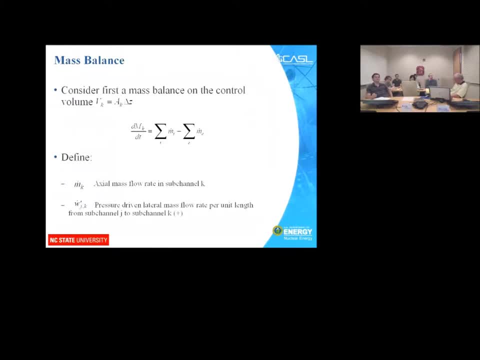 would be sub channel K, maybe axial location I in contact with sub channel J location. I in contact with sub channel J location. I in contact with sub channel J. so there's all of this and I'm not going. so there's all of this and I'm not going. 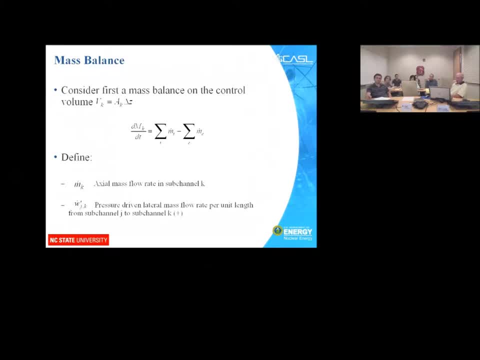 so there's all of this and I'm not going to include all of that again. it can get to include all of that again. it can get to include all of that again, it can get. it can get confusing enough with just a. it can get confusing enough with just a. 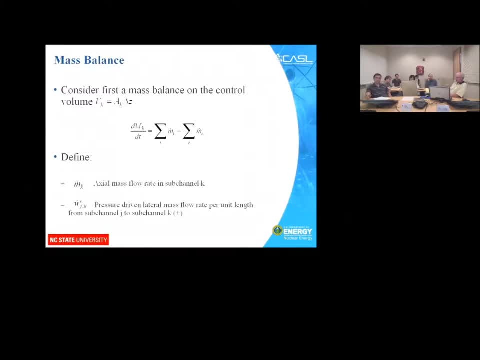 it can get confusing enough with just a subject with just a nomenclature. we'll subject with just a nomenclature. we'll subject with just a nomenclature. we'll have here but this when you see us. okay, have here, but this when you see us, okay. 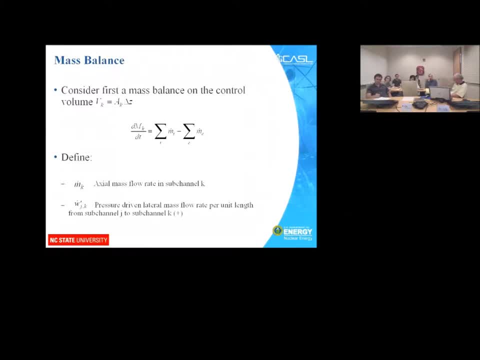 have here, but this when you see us, okay here. this means this is the sub channel here. this means this is the sub channel here. this means this is the sub channel. okay. so it's, this is going to be a. okay, so it's, this is going to be a. 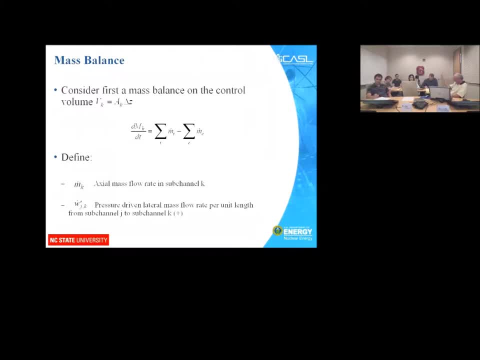 okay, so it's. this is going to be a particular sub channel that goes from particular sub channel, that goes from particular sub channel, that goes from the end up to the outlet of that sub, the end up to the outlet of that sub, the end up to the outlet of that sub channel between a number of rods in the 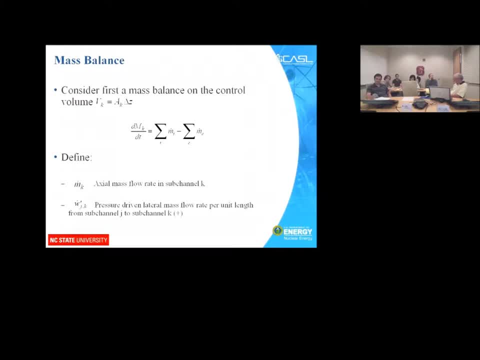 channel between a number of rods in the channel between a number of rods in the bundle, and so we'll denote the volume of bundle, and so we'll denote the volume of bundle, and so we'll denote the volume of that sub channel at any of that control. 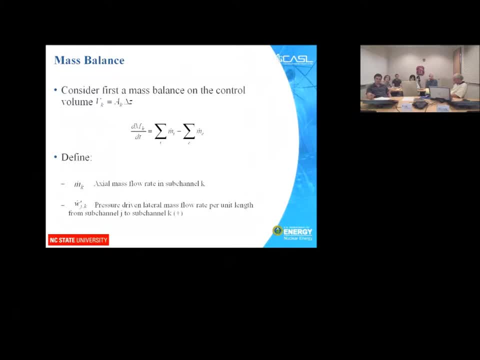 that sub channel, at any of that control, that sub channel, at any of that control, volume is just the area associated with volume, is just the area associated with volume, is just the area associated with sub channel, and this can be axially sub channel and this can be axially. 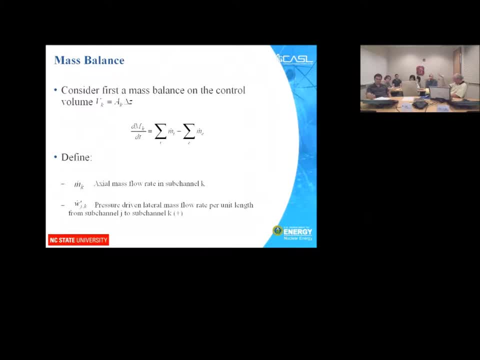 sub channel and this can be axially dependent, so the area can change as you dependent. so the area can change as you dependent, so the area can change as you move up the channel. so, for example, if move up the channel, so, for example, if move up the channel, so for example, if you have rods bowing, you can take that. 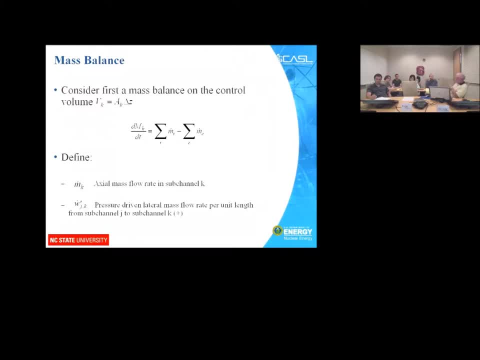 you have rods bowing, you can take that. you have rods bowing, you can take that into account if you would like. so the into account if you would like so the into account if you would like so. the volume of the that small control volume. volume of the that small control volume. 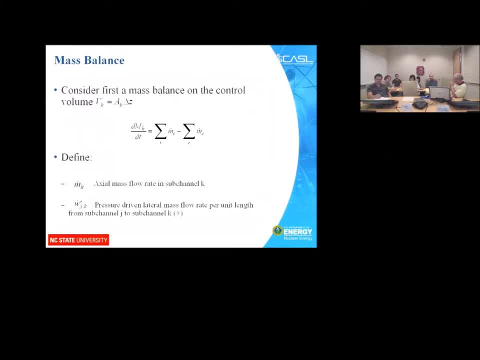 volume of the, that small control volume that I showed you in the previous slide, that I showed you in the previous slide, that I showed you in the previous slide, simply the area at that particular axial, simply the area at that particular axial, simply the area at that particular axial location. times some space deficit? okay, 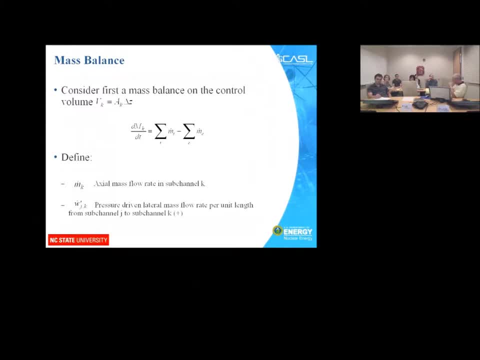 location times: some space deficit okay. location times: some space deficit okay. and the simple math out says that the. and the simple math out says that the. and the simple math out says that the time rate of change in the mass within, time rate of change in the mass within. 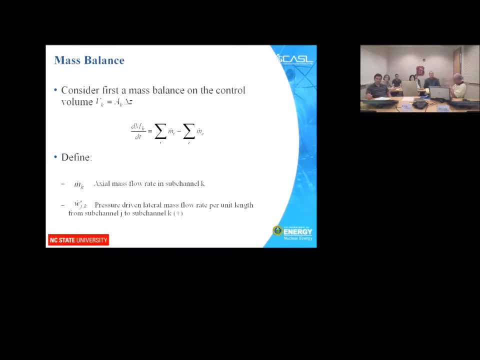 time rate of change in the mass. within that little control volume is the sum. that little control volume is the sum that little control volume is the sum over all the inlet strings of the max. over all the inlet strings of the max, over all the inlet strings of the max flow rates come in minus the sum over. 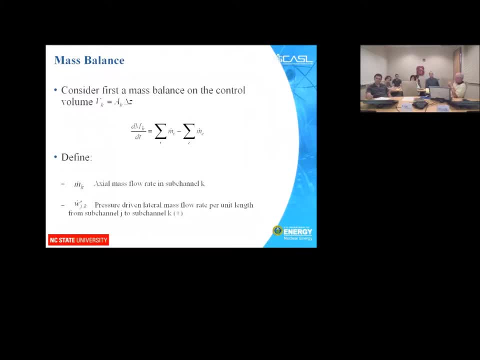 flow rates come in minus the sum over flow rates come in minus the sum over all the extra streams of the mass flow, all the extra streams of the mass flow, all the extra streams of the mass flow. racially so time ready to change is racially so time ready to change is. 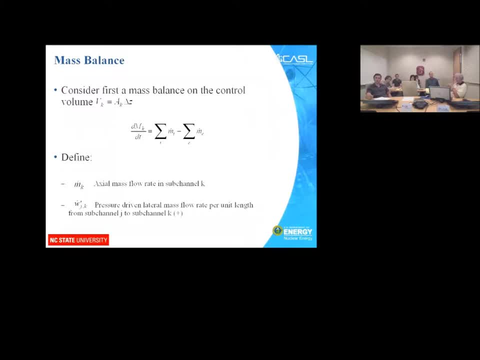 racially. so time ready to change is equal to what goes in minus what goes out. equal to what goes in minus what goes out, equal to what goes out. okay, that's it, and what we will then do is: okay, that's it, and what we will then do is: 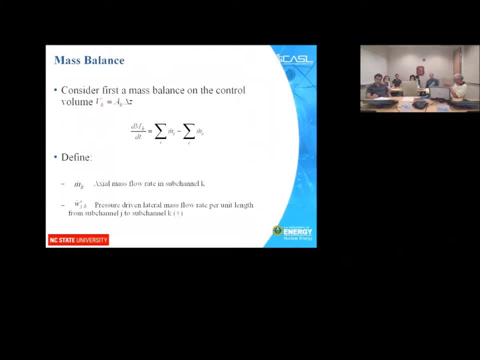 okay, that's it, and what we will then do is we're going to then look, remember we. we're going to then look, remember we. we're going to then look, remember we have two different, or we have several have two different, or we have several have two different, or we have several different kinds of flows got. 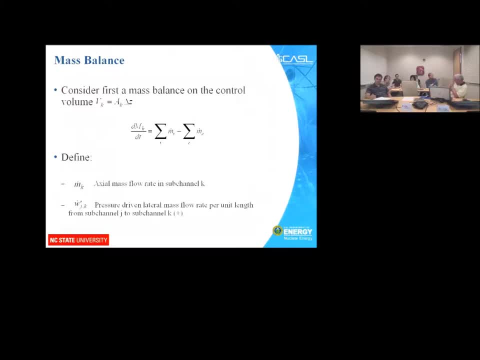 different kinds of flows, got different kinds of flows, got pressure-driven flows and we've got pressure-driven flows and we've got pressure-driven flows and we've got these turbulent mixing flows. you've got these turbulent mixing flows. you've got these turbulent mixing flows. you've got axial flows and lateral flows that are. 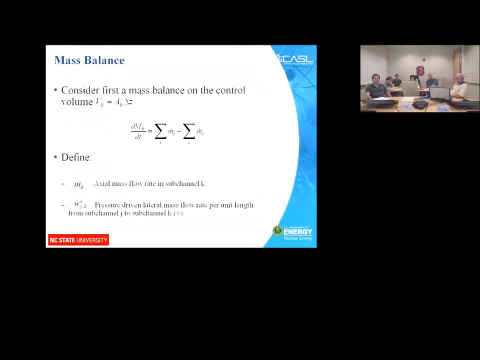 axial flows and lateral flows that are axial flows and lateral flows that are going to have to be included in these, going to have to be included in these, going to have to be included in these different summations. so the nomenclature, different summations. so the nomenclature. 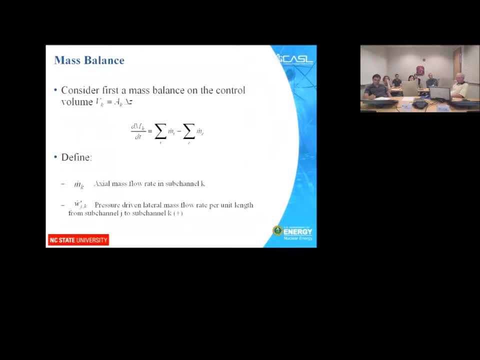 different summations. so the nomenclature that I will use is M dots of K. is the that I will use. is M dots of K. is the that I will use. is M dots of K. is the axial flow rate in sub channel K. so axial flow rate in sub channel K. so 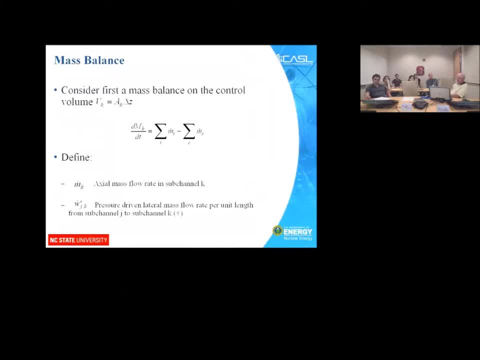 axial flow rate in sub channel K. so that's what's moving in the Z direction. that's what's moving in the Z direction. that's what's moving in the Z direction, and then there will be a the, and then there will be a the, and then there will be a, the pressure-driven lateral flows. what would 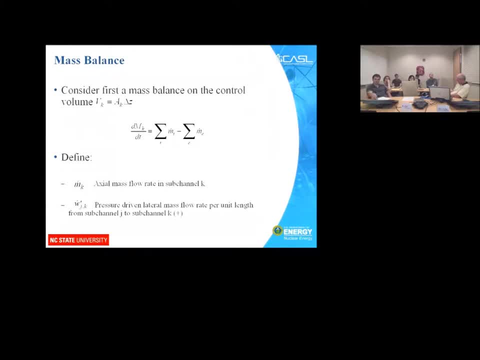 pressure-driven lateral flows. what would pressure-driven lateral flows? what would define is W dot prime J comma K and the define is W dot prime J comma K and the define is W dot prime J comma K. and the way that I do my subscripts is it's. 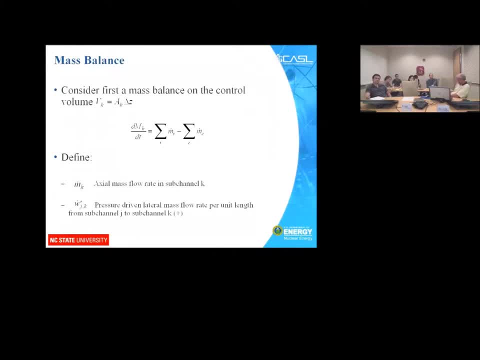 way that I do my subscripts, is it's way that I do my subscripts, is it's positive flow in the direction of the positive flow, in the direction of the positive flow in the direction of the subscript. so positive flow here would be subscript. so positive flow here would be. 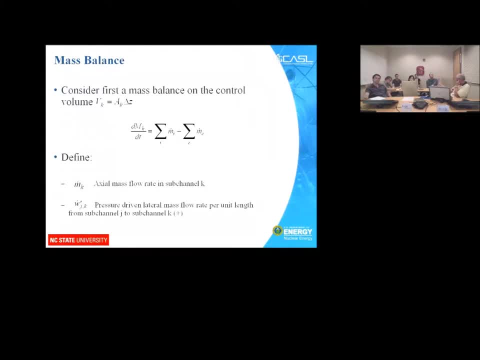 subscript. so positive flow. here would be W dot. this would be J to K. would be W dot. this would be J to K. would be W dot. this would be J to K. would be positive. so we would have positive flow, positive so we would have positive flow. 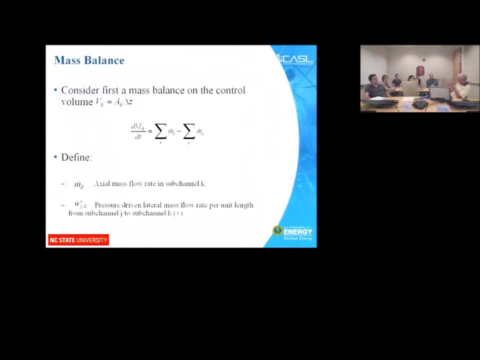 positive. so we would have positive flow here would imply that for sub channel K here would imply that for sub channel K, here would imply that for sub channel K we have flow coming positively from J, we have flow coming positively from J, we have flow coming positively from J into K. all right, and this is a, this is 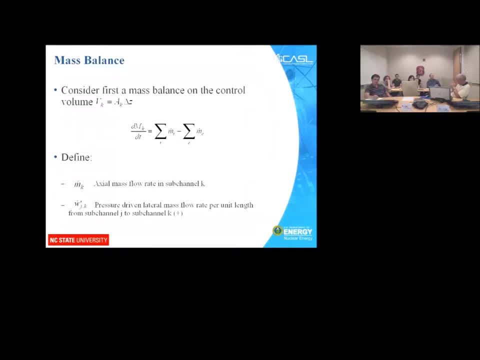 into K, all right, and this is a. this is into K, all right, and this is the pressure driven lateral flow per unit. the pressure driven lateral flow per unit. the pressure driven lateral flow per unit length. so this would be multiplied by a length. so this would be multiplied by a. 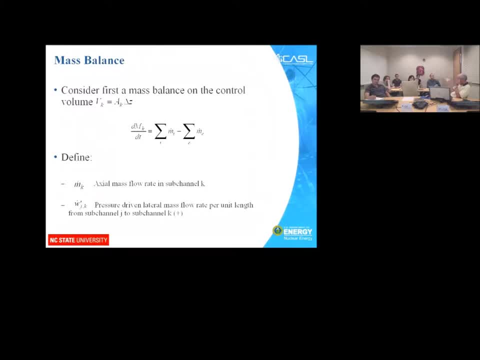 length. so this would be multiplied by a link segment to give you the total mass link segment, to give you the total mass link segment, to give you the total mass flow rate that's coming across that gap flow rate. that's coming across that gap flow rate. that's coming across that gap at that location. okay, so if we then go, 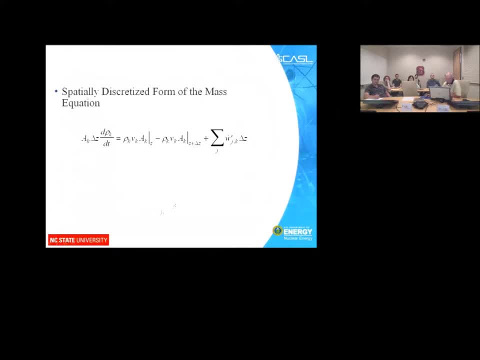 at that location. okay, so, if we then go at that location, okay, so if we then go ahead and just write this down, this then ahead and just write this down, this, then ahead and just write this down. this then represents the axial component, represents the axial component, represents the axial component of the flow. okay, what comes in? actually? it. 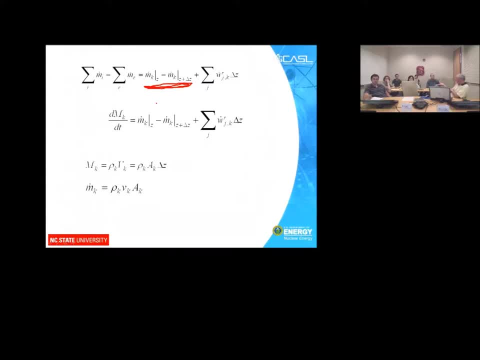 of the flow. okay, what comes in actually. it of the flow. okay, what comes in actually. it comes in at the lower limit of the, comes in at the lower limit of the. comes in at the lower limit of the sub volume. think of that as Z or if you want. 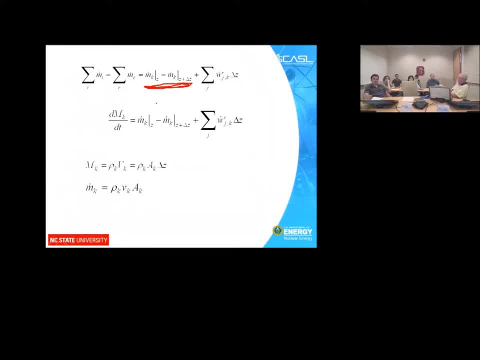 sub volume. think of that as Z. or if you want sub volume, think of that as Z. or if you want to think of it as a computational, to think of it as a computational, to think of it as a computational node, then you and in fact what you'll find, node then you and, in fact, what you'll find, node then you and, in fact, what you'll find, is that these equations going to, is that these equations going to, is that these equations going to look just like the axially discretized? look just like the axially discretized. 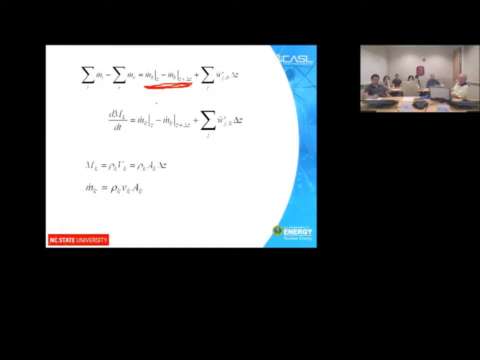 look just like the axially discretized equations, once we get done with them. equations, once we get done with them. equations, once we get done with them. okay, that's what they're going to look. okay, that's what they're going to look. okay, that's what they're going to look like. so this first term represents the 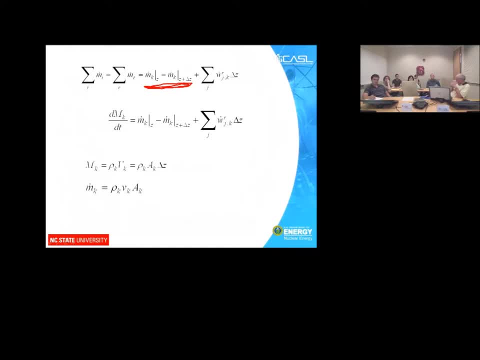 like. so this first term represents the like. so this first term represents the inflow and outflow in the axial inflow and outflow in the axial inflow and outflow in the axial direction of that control line, and then direction of that control line, and then 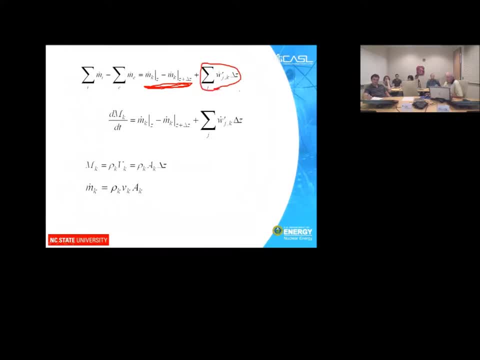 direction of that control line. and then this last term represents the net mass. this last term represents the net mass, this last term represents the net mass, transfer associated with cross flows and transfer associated with cross flows and transfer associated with cross flows. and again, this is with the convention that 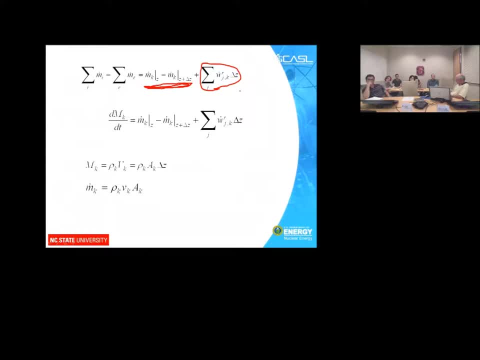 again, this is with the convention. that again, this is with the convention that I have shown here all of these flow is I have shown here, all of these flow is I have shown here, all of these flow is positive. these jk is positive, which positive. these jk is positive, which. 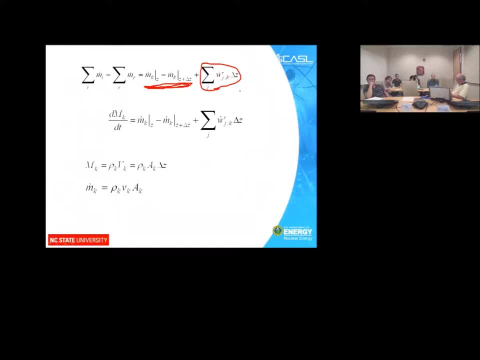 positive. these jk is positive, which means that if the flow is actually from means that if the flow is actually from means that if the flow is actually from K to J, it would be negative. so you just K to J. it would be negative, so you just. 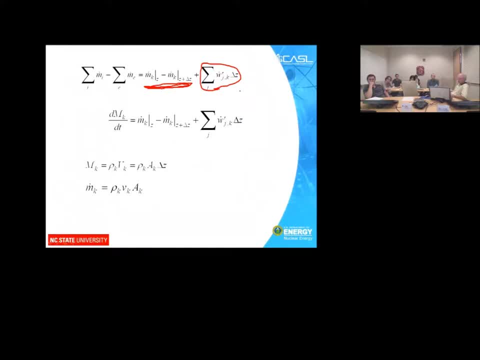 K to J. it would be negative. so you just put this on, okay, but this one. you'll put this on okay, but this one. you'll put this on, okay, but this one. you'll notice that there is no turbulent notice, that there is no turbulent notice, that there is no turbulent mixing term here, because, again, those 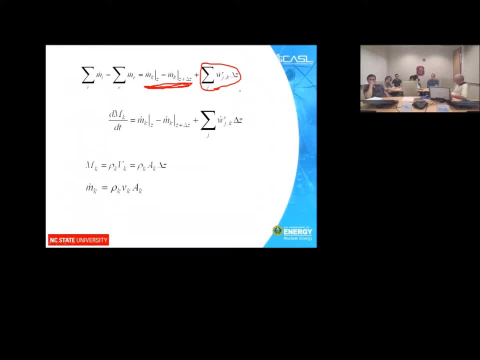 mixing term here. because again those mixing term here, because again those terms do not. there is no net mass terms, do not? there is no net mass terms, do not. there is no net mass transfer associated with them. so they do transfer associated with them. so they do transfer associated with them. so they do not appear in the mass equation. they 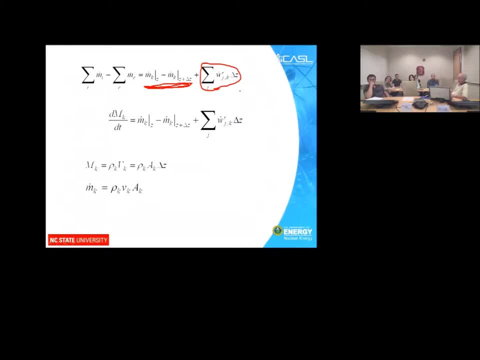 not appear in the mass equation. they not appear in the mass equation. they only appear in the energy and momentum, only appear in the energy and momentum, only appear in the energy and momentum equation. when we do those, you'll see. equation. when we do those, you'll see. 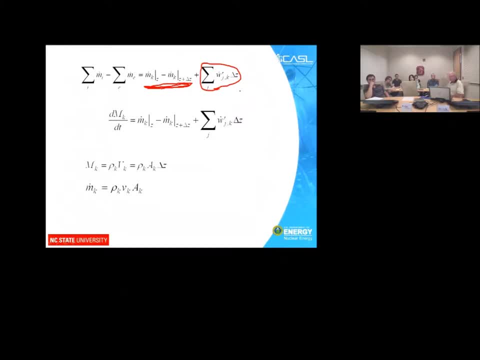 equation. when we do those, you'll see those there. so again I just this one's those there. so again I just this one's those there. so again I just this one's easy. so we simply substitute that term easy. so we simply substitute that term easy. so we simply substitute that term into our mass balance. and at this point, 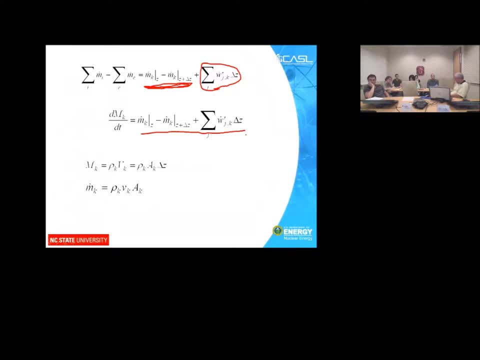 into our mass balance. and at this point into our mass balance, and at this point you're almost done. we cast things then, you're almost done. we cast things then, you're almost done. we cast things then into variables that we that are of, into variables that we that are of. 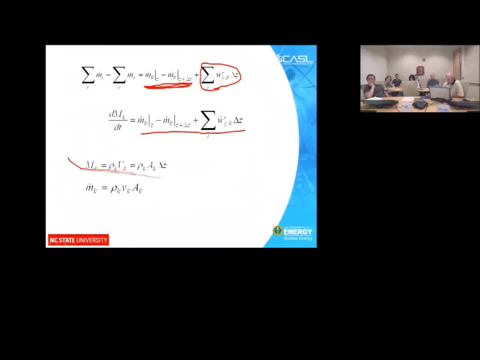 into variables that we, that are of interest. so we will rewrite the mass in interest. so we will rewrite the mass in interest. so we will rewrite the mass in terms of the density times, the volume terms of the density times, the volume terms of the density times, the volume, okay, and the mass flow rate in the 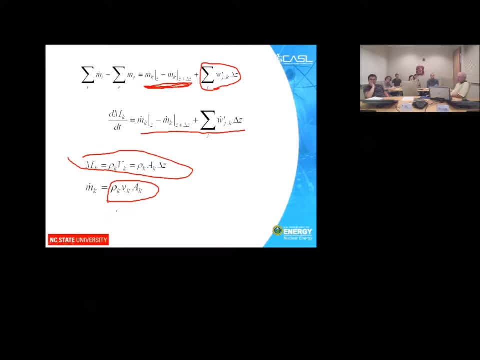 okay and the mass flow rate in the okay and the mass flow rate in the axial direction is the density times. the axial direction is the density times. the axial direction is the density times, the velocity v sub K, and again that is. velocity v sub K, and again that is. 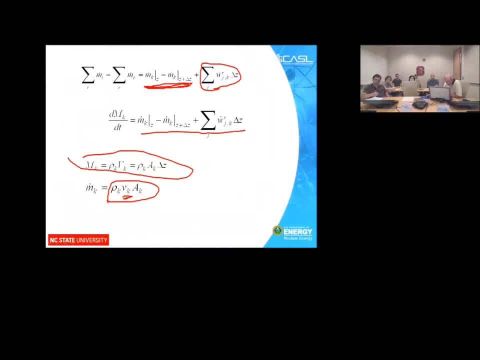 velocity v sub K, and again, that is that V sub K that I write here, is the. that V sub K that I write here is the that V sub K that I write here is the axial velocity, the velocity in the Z axial velocity, the velocity in the Z. 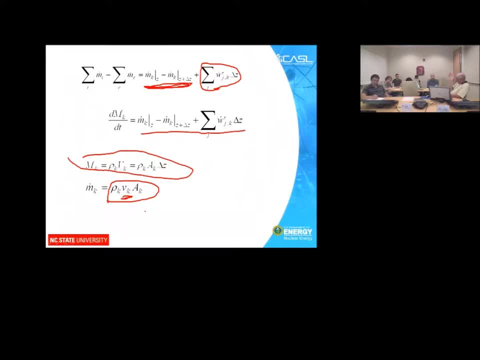 axial velocity, the velocity in the Z direction, in sub channel K, at the direction in sub channel K, at the location z that we happen to be working with. So I make those substitutions And you end up with what is the axially or spatially discretized form of the mass equation. 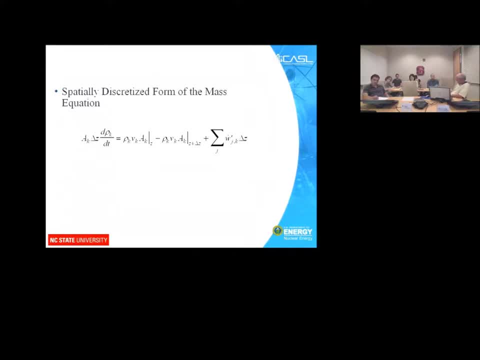 Now again, this applies at any axial node. So this would be the equation that would be solved at any axial location. So if you want to think about it, you can replace where I have z here or where I've got z plus delta z here, if you want to think of that as some i and i plus 1 and some axial. 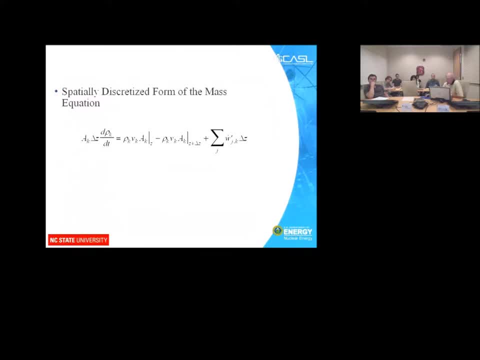 nodalization. that's what that would represent And the density that I have indicated- and I'll go here, this density, if you want to think about it, would have an i subscript on it also, So it would be subchaptered. 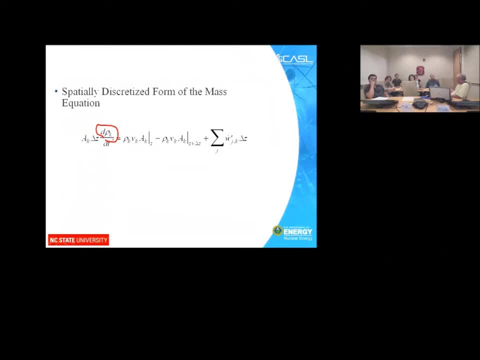 So it would be subchannel k, axial location. i Now what this looks like if you look at this equation, that term right there. if you divide that by the delta z, that looks like a standard first-order difference. And most of these codes, that is in fact I'm not aware of codes where they do not treat 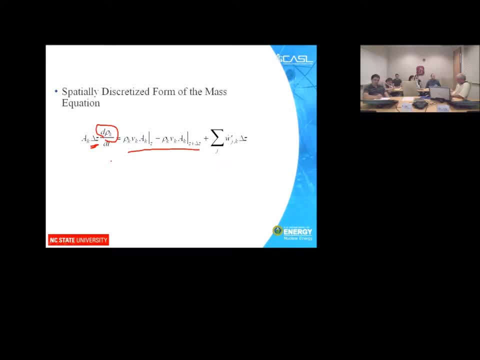 the axial discretization in this sort of form as a simple first-order difference, And that's the general difference type approach. okay, So that gives you some idea about error order for these codes. Okay, So they're all going to look at like a simple first order, okay. 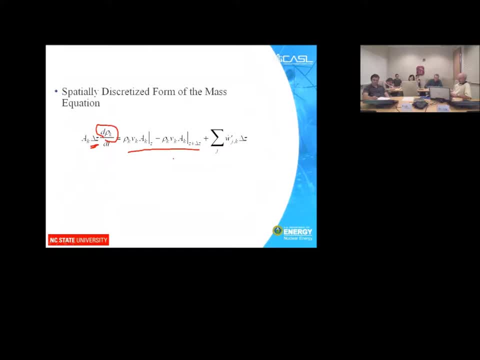 In this case, depending on how you, this would be a forward difference, Simple forward difference. Okay, So that's the mass equation, And the same approach is going to be applied to it. Now, in this case, this is something we'll talk about in a moment. 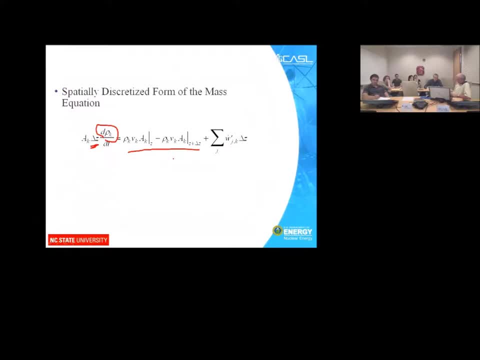 this equation there is nothing, there are no empirical correlations. So the only thing that would affect here is what spatial resolution you choose for your axial discretization will affect the solution and what the equation looks like for the prediction of that cross flow term. So if there are the impact of empirical correlations on this equation, are 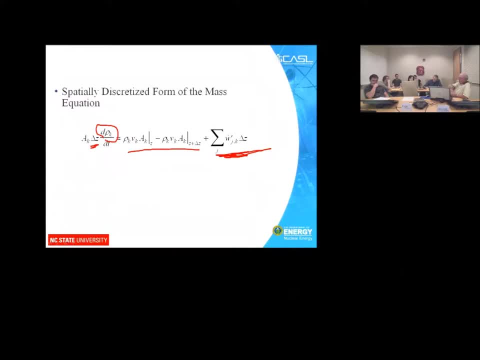 going to come only in the equations that are going to give you these additional parameters. So there's nothing in here. if you want to think about it, to adjust, I guess I'm not sure- the background of all of the people here, the energy balance, is. 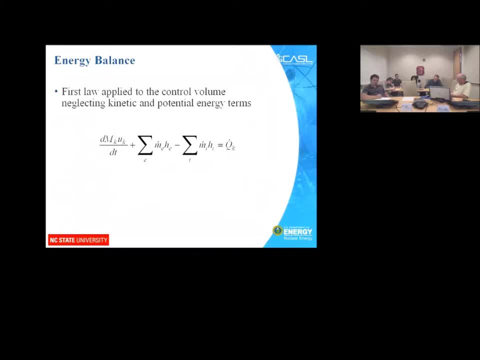 nothing more than a simple equation. Okay, So the energy balance is a simple application of the first law of thermodynamics that is in any junior level basic engineering curriculum. And the first law and most energy equations will have a kinetic energy term and a potential energy term, whether you're talking about 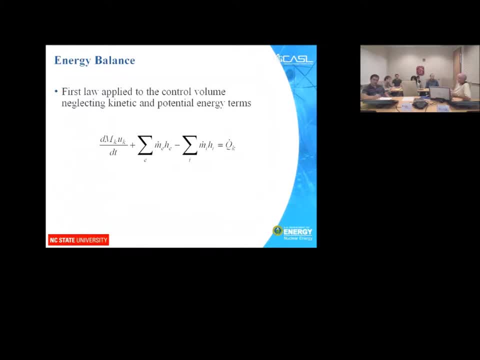 the first law or not, your studies or whatever, the energy equation will have those In engineering applications, particularly when you're looking at rod-bumble type geometries. the energy equation will have the kinetic energy term and the potential energy term And the second. 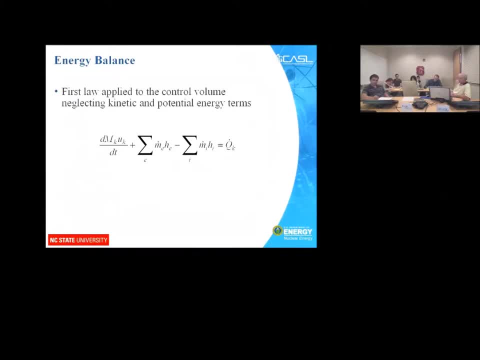 law is the kinetic energy term. When you're looking at rod-bumble type geometries, the kinetic energy terms are not significant. Okay, They just are not significant, And so they are almost always. In fact, I'm not familiar with any sub-channel code that actually includes. 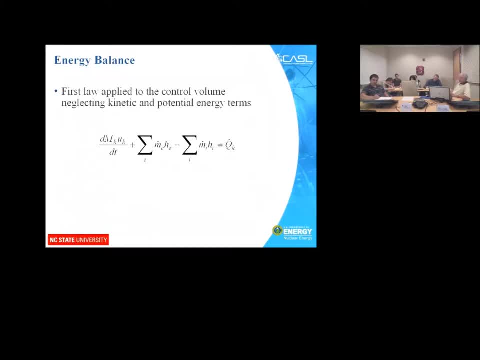 them. Those are neglected. So the energy balance is based on enthalpy, which is the H term here, internal energy and then the mass flow rates and so on that we mentioned before, And this term on the right hand side And this term on the left hand side is the 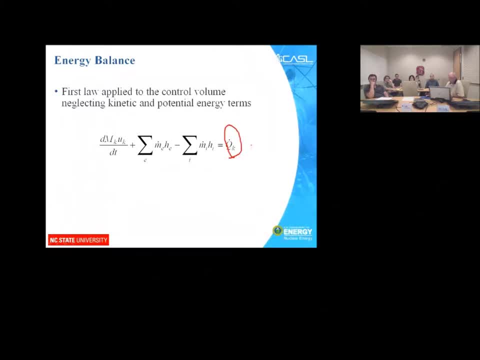 Depending on how you want to define it. that is the total heat addition rate to the subchannel, and it can include wall heat transfer, the wall that is transferred directly into the fluid across the heated surfaces. It can also, if you want, to include direct deposition of energy into the fluid at that. 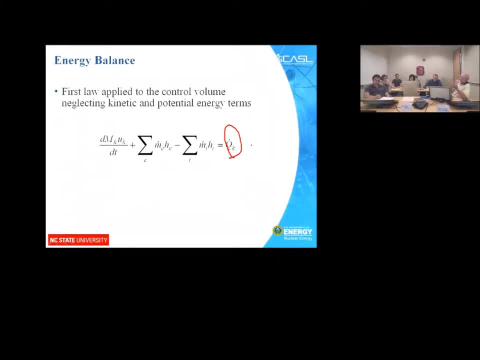 axial location from other sources, such as in neutronics. neutron thermalization inside the subchannel will directly deposit energy into the fluid at that location. You can include that in this term also. Okay, so it would have. if you want to think about it, it could have two different components. 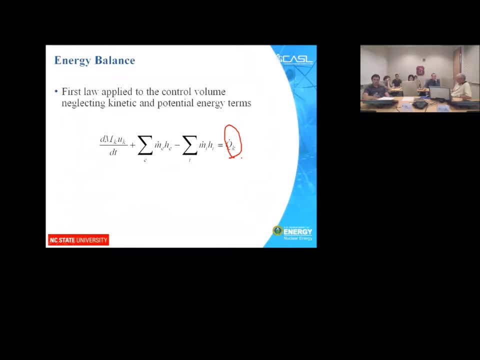 a wall heat transfer term and then an internal generation term associated with, again in neutronics it would be neutron thermalization. It could be chemical reactions that result in direct heating of the fluid, if you want to include chemical transport and chemical reactions in the fluid. 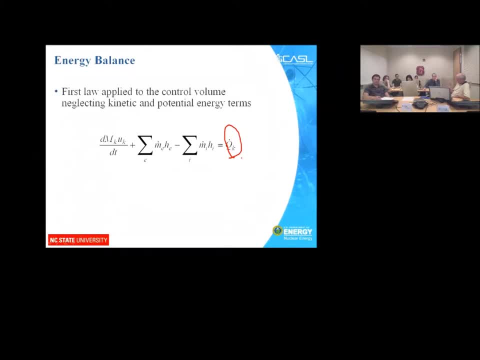 All of that can go in here For our purposes. for now we'll just assume that this is some heating term. if you're doing neutronics calculations, then the neutron transport will affect that, because if it calculates a neutron flux distribution in the coolant at that location, then that term could be. 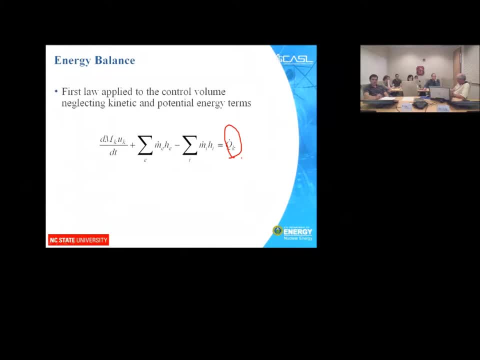 your volumetric heating term. that comes directly from the neutronics, So in that sense there's a direct coupling. In addition, the density distributions affect moderation, which impacts the neutron flux distribution. So all of these are coupled. If you're talking about this term having a wall heat transfer part, then that will be. 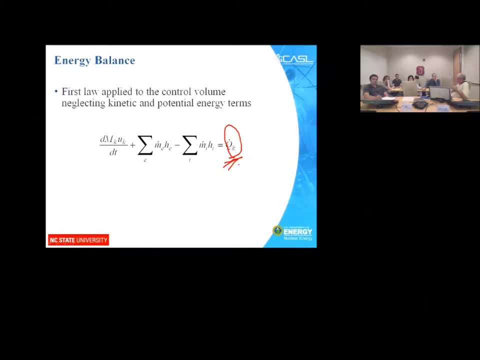 dealt with generally using empirical correlations, but could also, and it will involve- solving the heat conduction equation in heat transfer, Typically inside of the wad. it calculates what heat transfer is from that wad into the fluid across that heated surface. 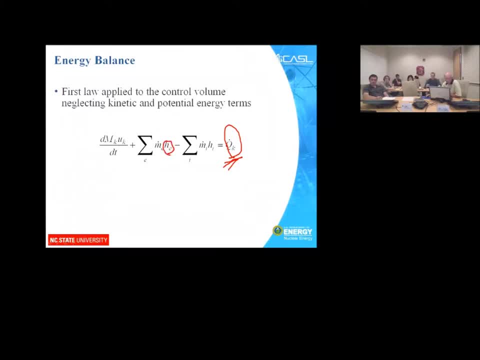 So the H terms here are enthalpy, The U term here is internal energy, and internal energy and enthalpy are related by basic thermodynamic relationships. The enthalpy is the internal energy plus the pressure divided by the density. So if you're not a school of thermodynamics, 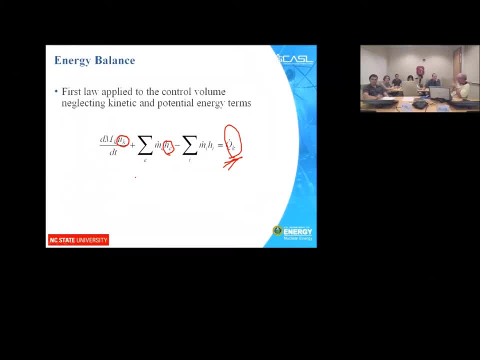 The enthalpy is simply this: U parameter plus pressure divided by density. Pressure and density will show up in the equation later on. So the convective terms have three components. We've already seen two of these in the previous slide. One is the axial flow component. 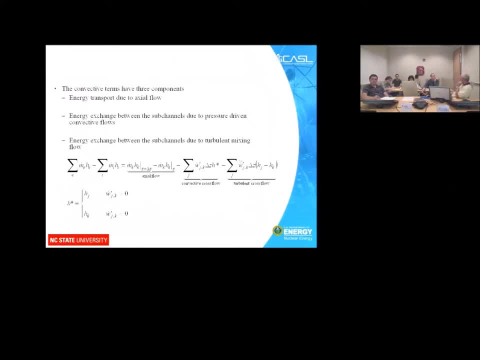 It's going to show up, And so that one we've dealt with the math equation, We have the energy exchange between the subchannels as a consequence of the pressure-driven convective flows, So that one also that mass flow rate, that pressure-driven convective flow we saw in 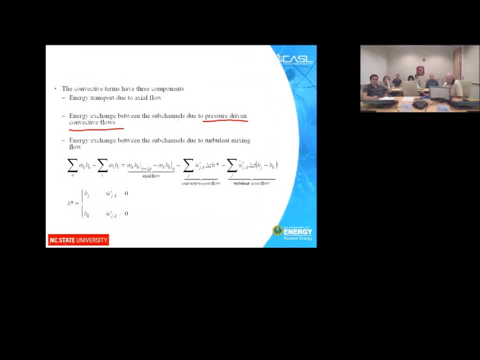 the mass equation also, but then we've got the additional turbulent mixing term, which did not appear in the mass equation but does appear here now, And so, without me going through a lot of details, I'm just going to show you a little bit of. 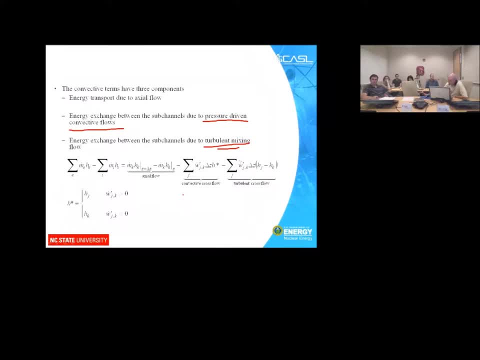 the flow parameters, And if you're wondering what this is, we are going to use the horizontal flowilton, which we'll talk about here in a moment … … … …. However, it may not be exactly the μποutFT … …. 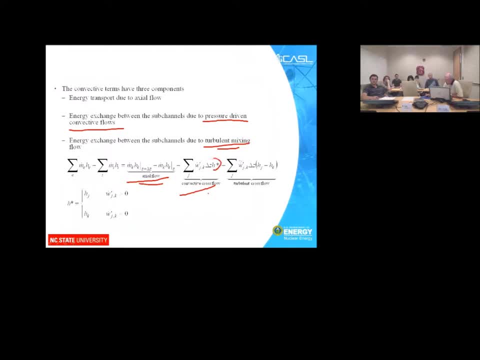 … …, … … … … … … … …. mAcA …. mAcA, faktInfl commute of the infl towards. 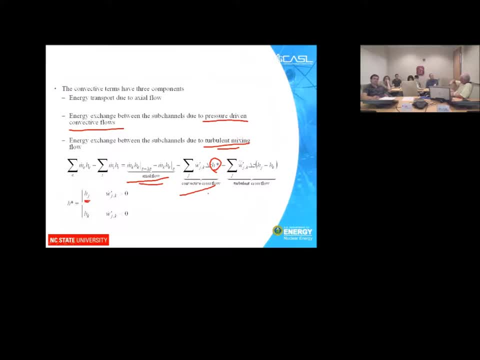 marketers choice across the protections. awkward how to figure out this. Bedford is for the fan with the SUN clear preach max, such as channel J into sub-channel K. it would be the enthalpy in the sub-channel K if the flow is out of the sub-channel. 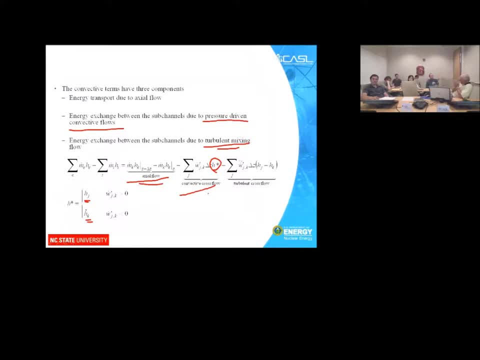 So the convective flow carrying enthalpy into and out of these sub-channels across that gap is assumed to carry the enthalpy of the sub-channel, of the adjacent sub-channel, at that same axial location. That assumes, effectively, perfectly mixed, perfect mixing inside the sub-channel at that. 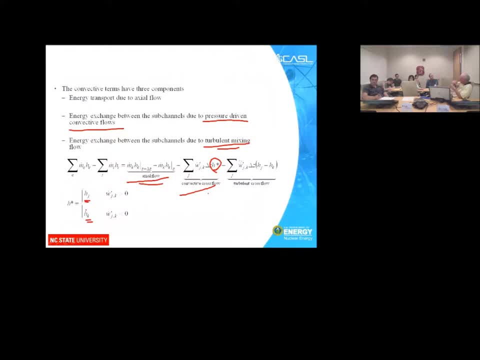 location. There are no spatial distributions assumed for the enthalpy distribution in the channel And again, this is another first-order type approximation for the transport across that boundary. Okay, So it's consistent with the spatial difference, at least in the axial direction. 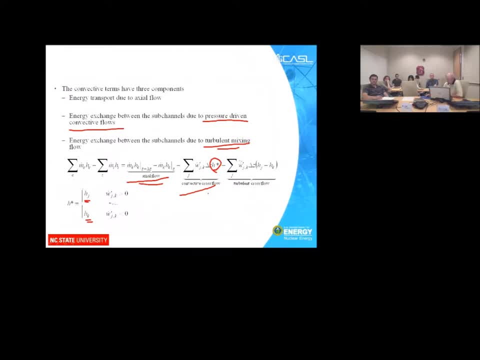 So the choice of which one you use is based on the sign of this: pressure driven Okay And the turbulent mixing term okay assumes again there's no net mass transfer. so whatever flows into the sub-channel in the mass sense again flows out again. but when it flows, 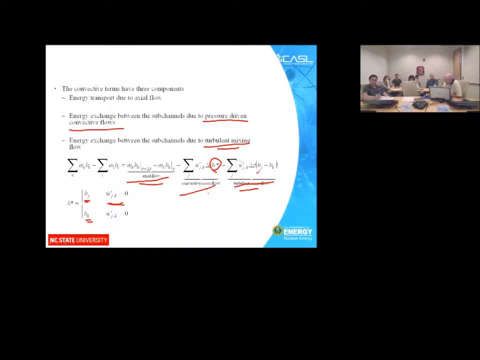 into the sub-channel, it carries with it enthalpy HJ, And when it flows out of the sub-channel, it carries with it enthalpy HK. Okay, So as it swirls in and out again, it carries in one enthalpy, it carries out another. 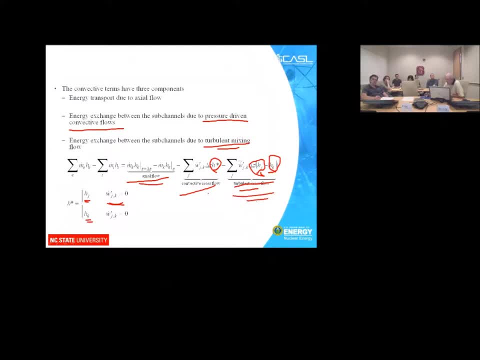 And so the effect of this term, even within the absence of any convective cross-flows, is to cause the channels to equilibrate in terms of enthalpy. If you had an infinitely long channel, then eventually what would happen was that everything. 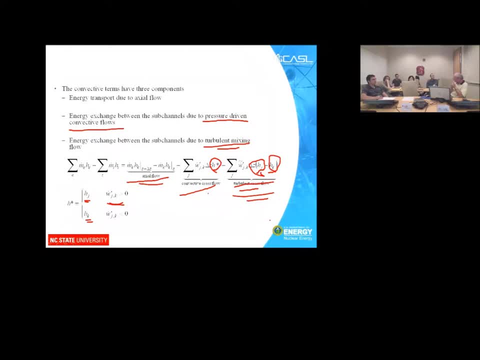 would come to the same enthalpy distribution at the axial as a consequence of this. Okay, This turbulent mixing term here, That turbulent mixing term, This turbulent mixing cross-flow, is an empirical parameter. okay, that is based on empirical correlations. 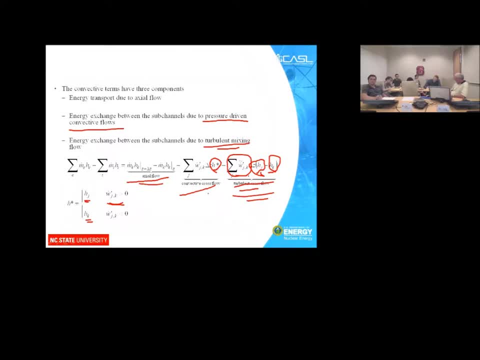 That thing is something that you will have, generally. a choice of the model one. what turbulent mixing model do you want to use? all right. And then there will be parameters within that correlation that can be adjusted. Okay. Now whether or not you have access to them is a different issue, but at least you know. 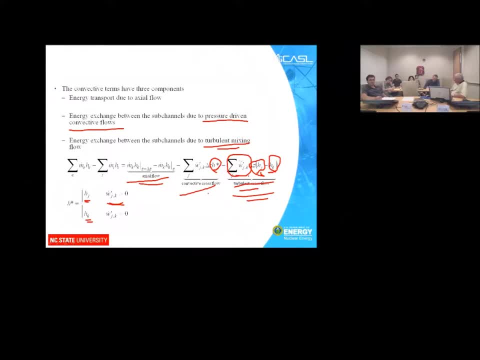 if you were looking for something to play with. okay, this is the first parameter that we have seen in terms of empirical correlations that you would be able to adjust. It's based on empirical data, measured data, Okay, And how do they determine it? 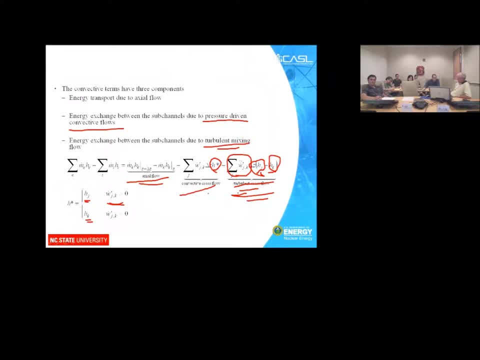 They run the sub-channel codes and they compare this, and so the sub-channel code itself is some large nonlinear, nonlinear, nonlinear, nonlinear, nonlinear, nonlinear, nonlinear, least squares model, and then they fit this model, they adjust that parameter or find. 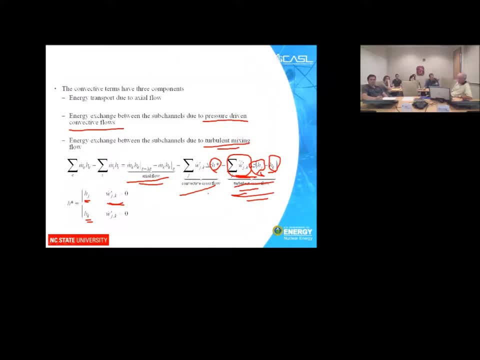 a form of that mixing term which gives the best fit for experimental data within the sub-channel code that you happen to be running. Okay, So the sub-channel model itself is your large nonlinear equation. if you will, that you're doing, let's say, a least square spin on and that's your fitting coefficient. 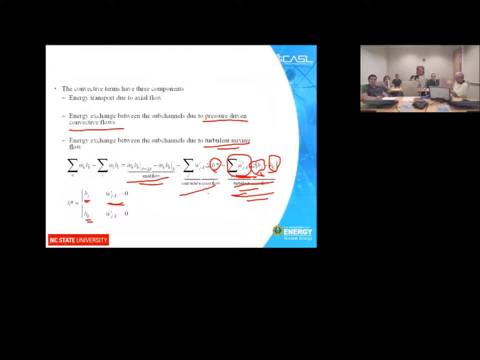 Okay, That thing, right, there is your fitting coefficient. That's how it's determined in general, is how they find these things Okay. So again, what that leads to is- and I've gone ahead and done the variable substitutions for mass, flow rate and mass to put this in form, so that again is you're spatially. 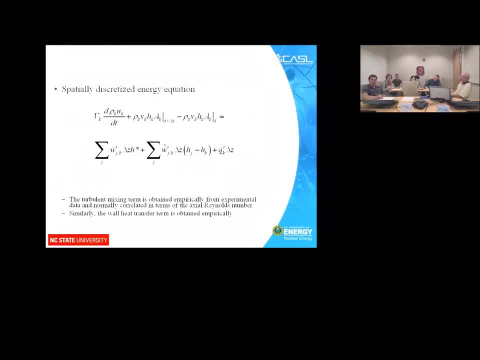 discretized, and this is discretized in the axial direction for the energy equation And again the, The parameters of that you have. that would be, for example, adjustable for people who are interested in uncertainty quantification, sensitivity analysis would be that one. 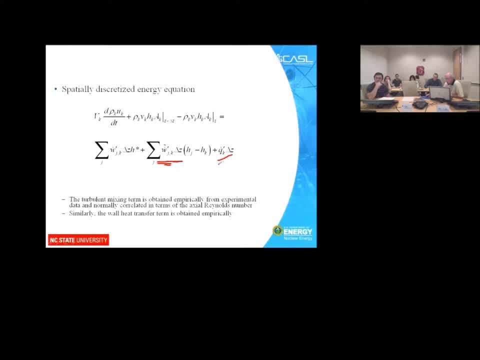 And then the other would be: let's assume that this term- and I've broken the heat transfer rate up into a heat transfer rate per unit length times a length, Okay, And so that term right there. Okay, If you want to think of it as being the wall heat transfer term, that thing would involve: 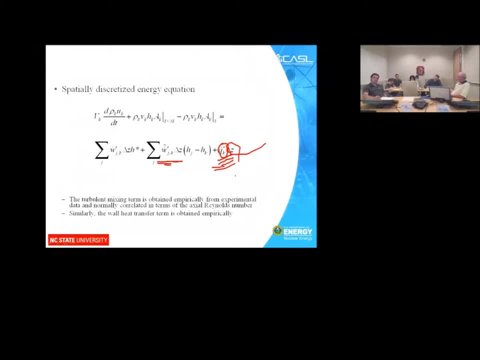 empirical correlations. Okay, And I have noted that in the little comments down at the bottom of this slide. The turbulent mixing term is obtained empirically from experimental data and it is normally correlated in terms of the axial Reynolds number. Okay, So the axial Reynolds number is that Reynolds number based on the axial velocity and the 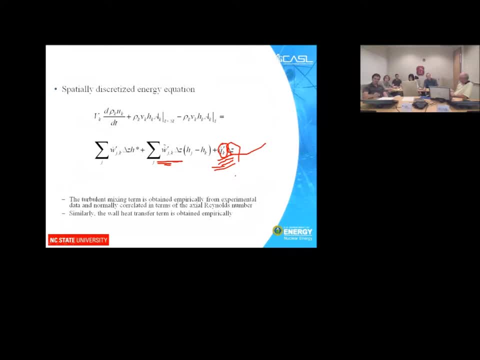 correlation is, in general, it's based on that Reynolds number- Okay, And again, it's empirically determined. And similarly the wall heat transfer term, the one I've indicated here, okay, that term will be. They will involve heat transfer coefficients that are based on empirical data. 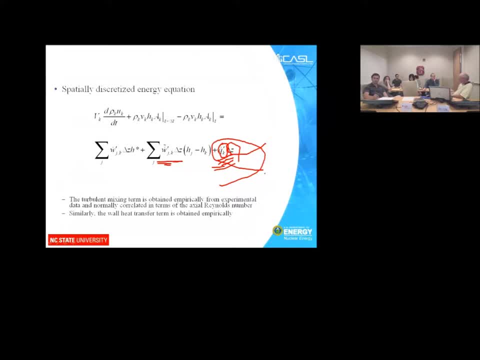 Okay, So Okay, And there will be different heat transfer coefficients depending on the heat transfer regime that you're in. So, for example, if it's single phase force convection, only there will be one correlation. If it is mixed boiling, where you have single phase force convection and nucleic boiling, 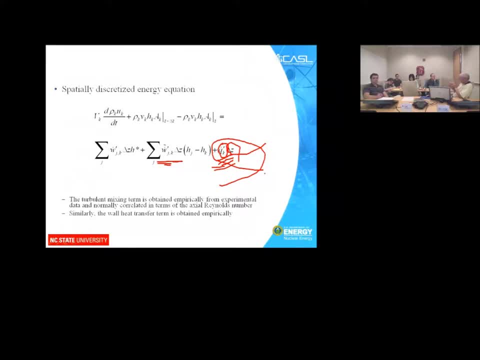 there will be some combination or some other correlation, And then, if it's simply boiling, then there will be a third correlation. still Now, in the current- Okay, In the current version of Cobra TF, the one that we're using, there is one correlation. 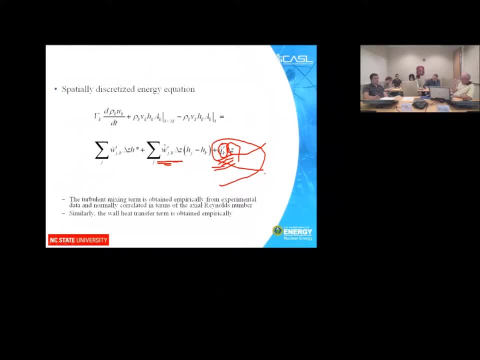 only that models heat transfer over the entire length and it's called the chin correlation. The problem with the chin correlation: it is not applicable to the flow regimes that we're interested in in CASL, So at some point that correlation is going to. 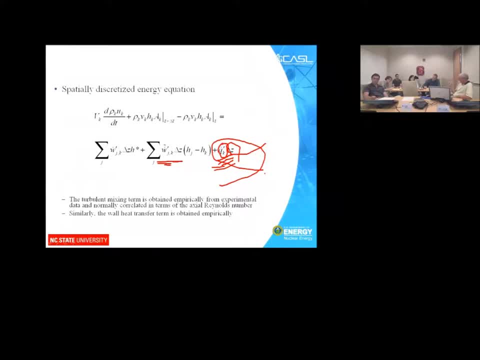 It is the only one that is in Cobra TF now, so you cannot choose correlations. There's one, chin, Okay, And so it's hardwired. There is no option for anything other than chin in Cobra TF right now, whether it's applicable. 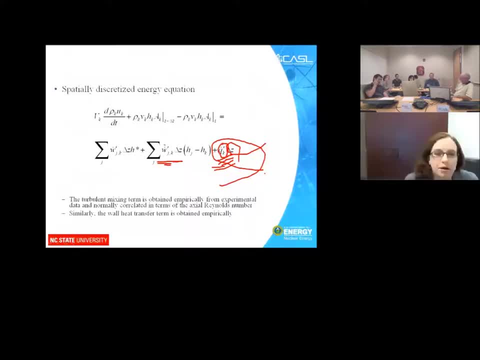 or not, And chin is applied over the entire rod bundle. Now the nice thing about chin is that the chin correlation has You can turn on and off. Okay, You can turn on and off different turns of it so that you can use it in the single-phase. 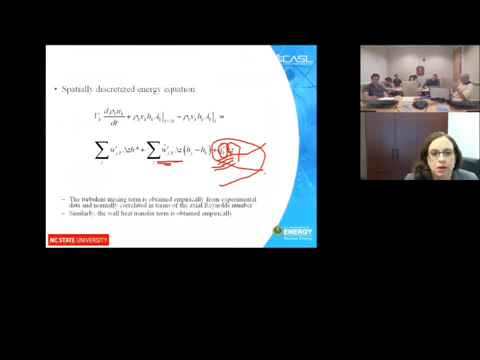 force convection region and in the boiling region. but you can't choose other correlations. You have no choice, and you don't have any choice as to how that one is implemented. Okay, And so there's nothing to adjust in that. 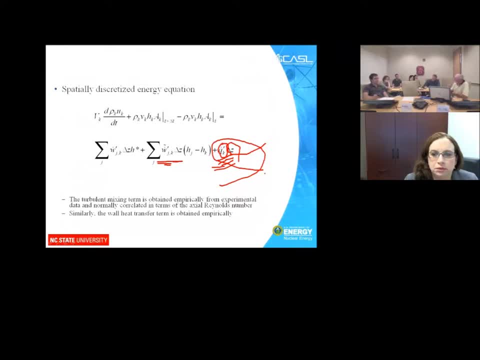 Well, if you want access to it, you've got to get access to it through the code itself. Okay, There's no other way to deal with it. Okay, All right, In the interest of time, I'm going to move forward. 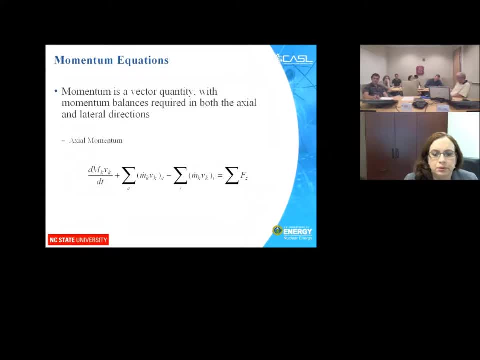 The momentum balance looks very, very similar to the energy balance You have, And you have two of these. We're going to have an axial momentum equation and we're going to have one in the lateral direction. The axial momentum equation is what's going to give you the pressure distribution in. 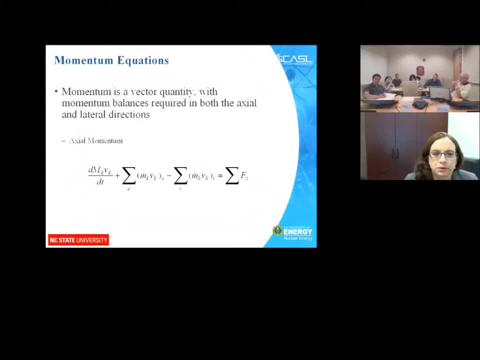 the axial direction And the lateral momentum equation is going to give you, Given an axial pressure distribution in adjacent subchannels, then how do you get the lateral flows as a consequence of that? So the axial momentum equation says simply that the time rate of change of the axial 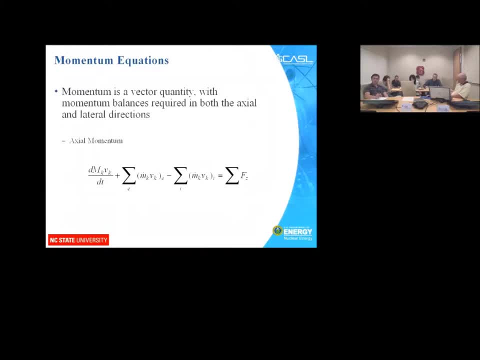 momentum is simply the sum of the inlet flows of momentum in the axial direction, minus the outlet flows, plus the sum of all of the forces which act on the fluid in the axial direction. All right, So that's going to give you a very similar pattern. 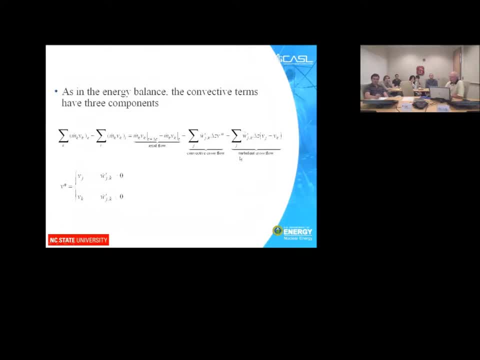 And let me I'll go ahead and move through this And again, we're going to have three components. You're going to have the axial flow component, You're going to have a convective crossflow component And you're going to have a turbulent crossflow component. 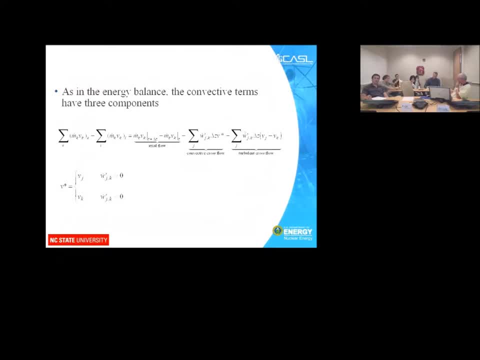 And if you look at the form of these terms, they look just like the energy equation, where now, instead of having amplies, I've got velocities. That's the only difference. And again, in this one, the, And even the way that you do it, is always the same. 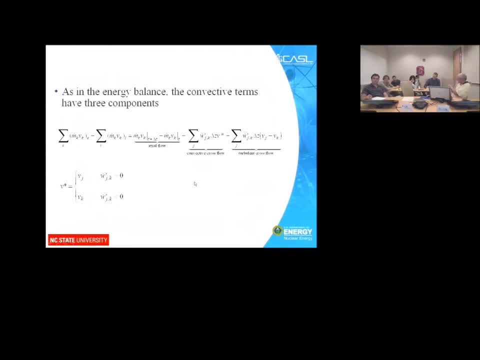 You're not going to be able to be in that particular location. you determine which velocity is connected from one channel to the next. it looks just like we did with the enthalpy inflation. So if you look at this there, for example, I put: 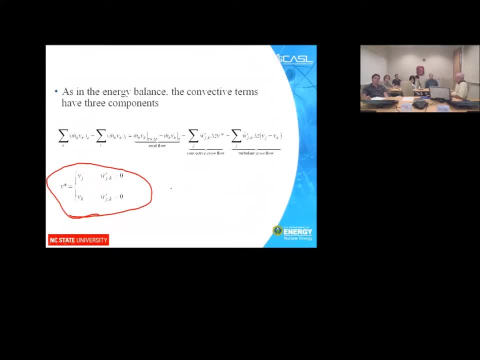 velocities instead of amplitudes, but that's the way it's typically done And if you look at the turbulent cross flow, it's done exactly the same way. So the same turbulent mixing term is there And one option that- and I think I'll make this comment- We'll come back. 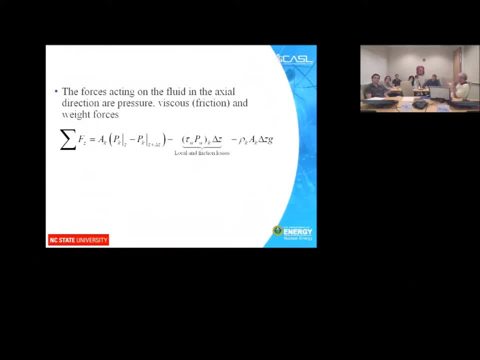 to that in a moment. So anyway, the form of that term is exactly the same as the energy transform term. You just put velocity in there instead of amplitudes, And then the forces that act on the fluid. you have pressure, you have energy, you have energy and you. 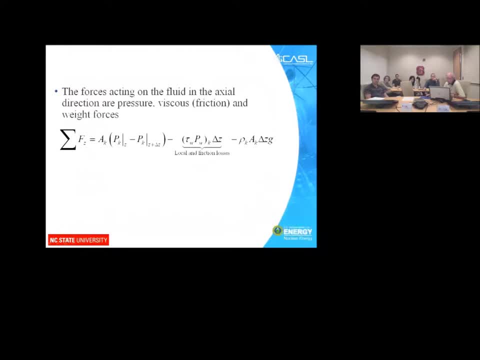 have pressure forces, okay, which are represented in terms of the pressure distribution axially in the channel. You have wall drag or frictional forces, While I'm not. this is another place where there are correlations. Okay, this is the place where there are correlations. 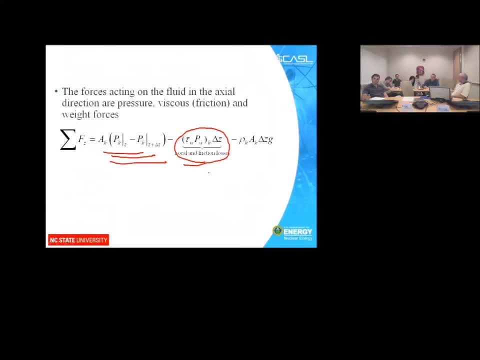 This is local losses are things such as entrance and exit losses, losses due to space. Okay, M. I mean, yeah, M. Yeah, many of you are already familiar with the loss as such. M, Yeah, definitely M, And we have the basic roots which we certainly have in these rod-bumble designs And there. 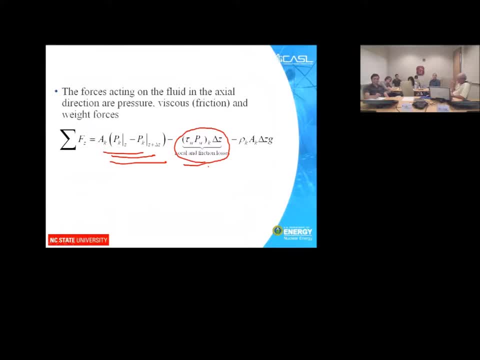 value for the grid. is that correct? Yes, Okay, so at n you specify at what axial location these the grid is. you input a fixed- it's called a K value or local loss coefficient- for that grid. okay, and it is treated as a discrete discontinuous. 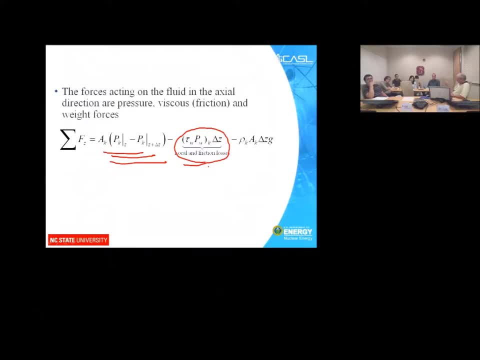 change of pressure at that location. okay, which says something about a link scale, because grids would be a couple of inches long maybe, but this occurs at a point. so there will be a step: discontinuity of pressure at that location as a consequence of this local loss coefficient You do have access to. 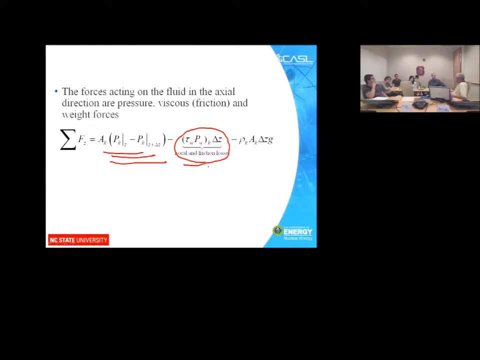 those. You can fiddle with it as many as there are spacing grids, okay. so there will be one loss coefficient per grid and you do have access to them through the input file, okay? The other component of the frictional loss is the continuous. 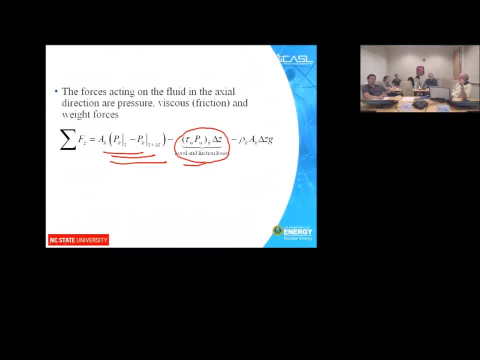 friction component, that is done by a friction controller. friction factor correlation, which again is in terms of the axial Reynolds number, And that one I don't believe you have any options on in Cobra TF. It is a given correlation. If you want to play with it you've got to go in and change the actual physical code. 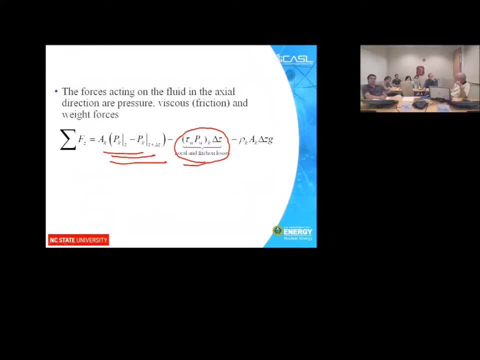 You cannot choose which one it is. You can't even choose the coefficients that are in it, And then you've got a weight term and that's just your axial, your buoyancy term. All right, so you put all that together, okay. 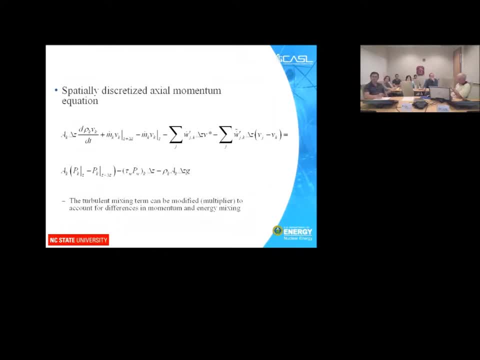 and then again, this is just the spatially discretized form of the axial momentum equation where these empirical terms show up again. You've got the turbulent mixing correlation. You've got friction and local losses, which will appear here and it will be correlated. 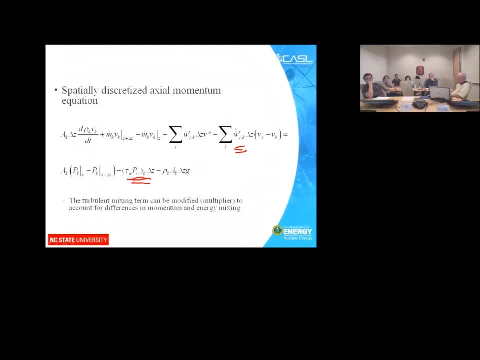 And again, you will at least have access to the local loss coefficient. And one thing that you will find in some codes is there is a distinction between turbulent mixing momentum transport and turbulent mixing energy transport, And in some codes they offer the option of modifying that term right there by a multiplier. 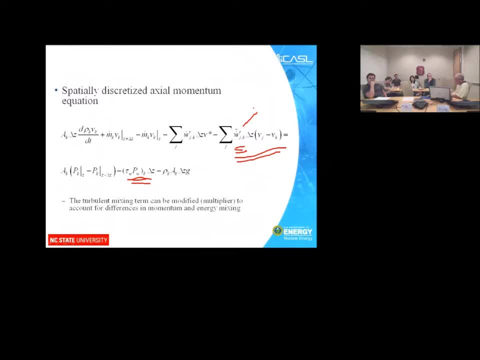 I do not know whether Cobra TF has that as an option. I'm not Okay, but you will see that in some codes. So what they'll do is they'll just take the turbulent mixing term and say, okay, there's a momentum multiplier. 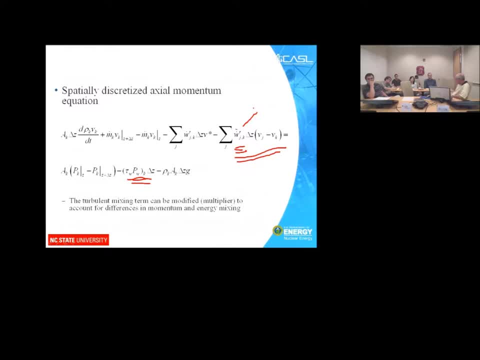 Okay, and so if they have that as an option, you might have access to that through the input. All right, All right. Now the last thing is the lateral momentum equation. Okay, since we have these lateral cross flows that are given that are the result of pressure differences at an axial location. 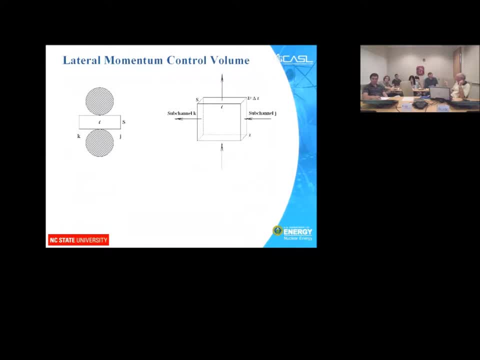 that is determined by performing a momentum balance across the gap between the two subchannels, And this is going to be written in terms of y. but y here is simply an arbitrary lateral direction. It is not a y coordinate. Okay, So do not confuse. 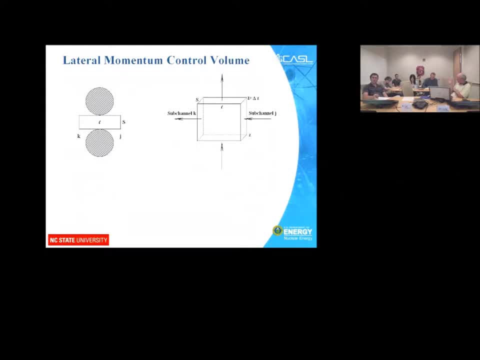 If you're locked into thinking x, y, z coordinates, do not. Y is simply an arbitrary direction from subchannel j to subchannel k and it could be pointed in any direction. It's just in the radial plane. Okay, So it could be pointing up sideways, crossways, whatever. 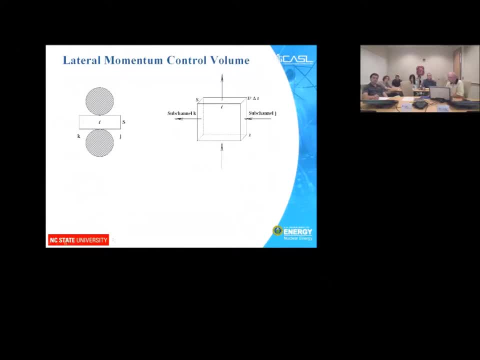 Whatever, it is Okay. So do not confuse y with actual y coordinates. It's not Okay. It is simply the direction laterally, And so you have a lateral momentum control volume and most of the time- and you can do this more advanced- 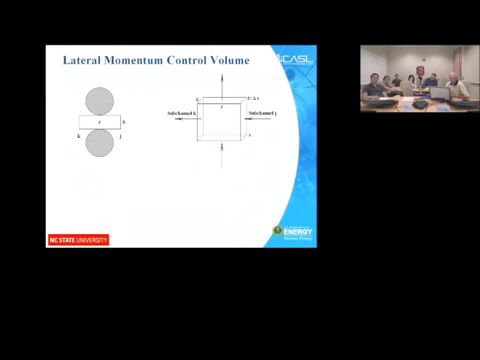 but this is fine using a box. The lateral control volume is simply indicated here and it is a square or it's a box. okay, as indicated here. Okay, And this is the center of subchannel k and this is the center of subchannel j- out here. 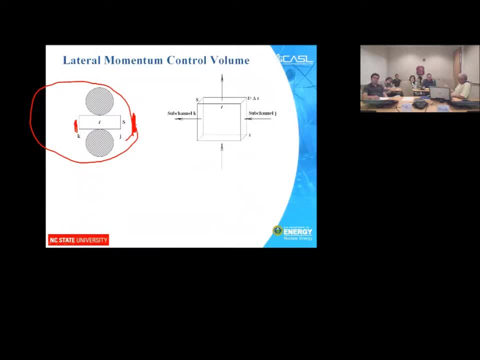 And you can point this lateral momentum balance in any direction necessary. That's why it doesn't matter whether it's a rectangular lattice, a triangular lattice or whatever, because each of the transport across any particular gap is assumed to not impact the transport across any other gap. 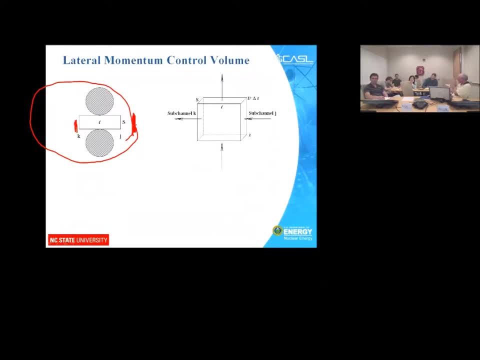 Okay, So once you have moved flow from subchannel j to subchannel k, if you go to another gap, it does not know that that transport has happened other than whatever the pressure is in this particular subchannel. So there's no j to j, if you will term. 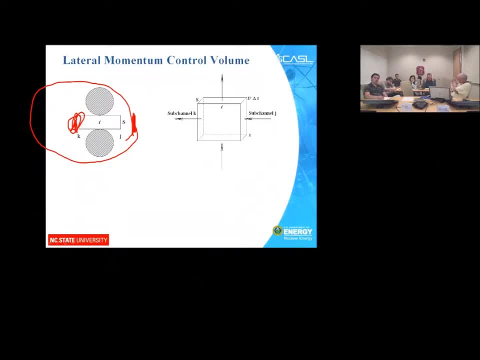 So you can't have a crossflow term which goes all the way across the subchannel to another subchannel. Okay, Once you cross into subchannel k, the fluid loses any idea of where it came from, And so, again, that allows you to write these balances. 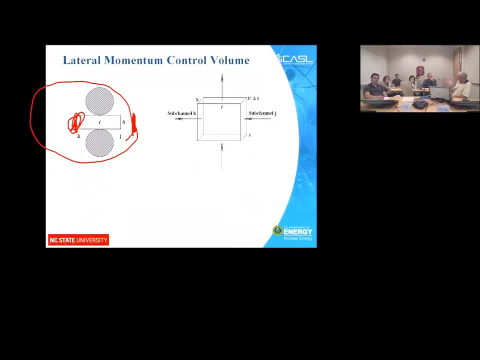 across each gap. And so again, we assume that the flow is from subchannel j across this gap into subchannel k And again the pressure, the center of subchannel k would be here and would have pressure pk. The center of subchannel j would be located here. 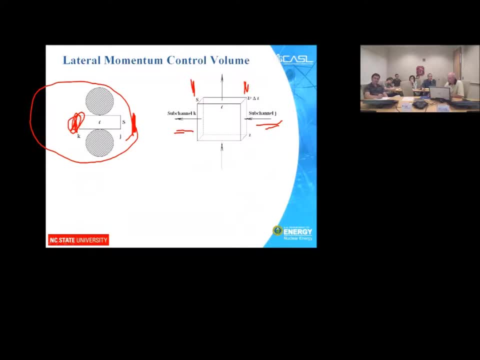 and have pressure pj And the momentum balance looks exactly the same as for the axial momentum, except now we've subscripted with y. Again, y is not a coordinate direction, It is simply a pointer, And the mass now is based on the volume of that box. 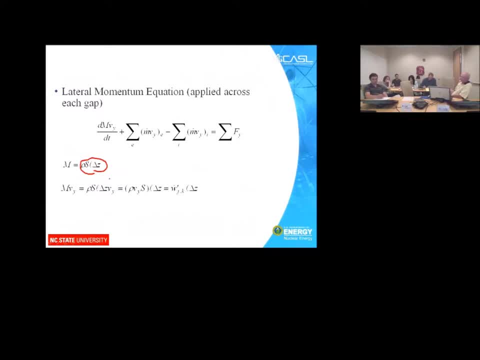 So the volume is the gap, spacing times, the center-to-center spacing L between the subchannel, and then the space, the width, And this does not have in it, if you look at this lateral equation, nowhere in it does it have the lateral crossflow term. 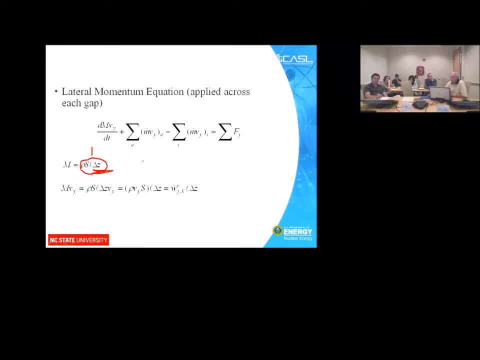 w dot prime jk. That doesn't appear in here. So we have to convert these things and these things into the lateral crossflow And if you expand them, you'll see that you have the lateral crossflow term w dot prime jk. 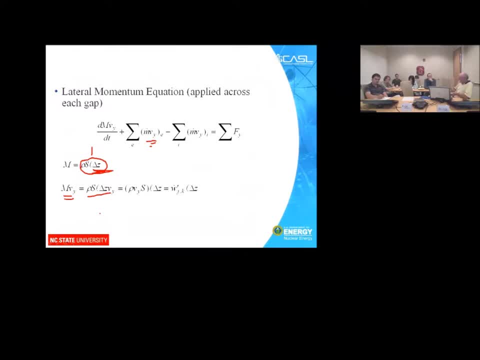 So if the mass again is written in terms of the density times, the volume of that box times this lateral velocity dy, and you group the density times the y velocity times the spacing s, then that by definition is the lateral crossflow per unit length. okay, 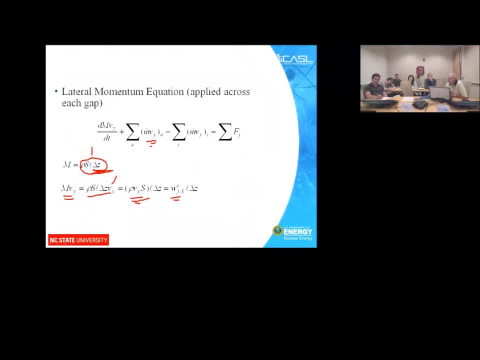 And we will use that then to convert all of these terms into the lateral crossflow. So, again, in the interest of time, let me move through these fairly quickly. We're about done, but let me go ahead and move through this. 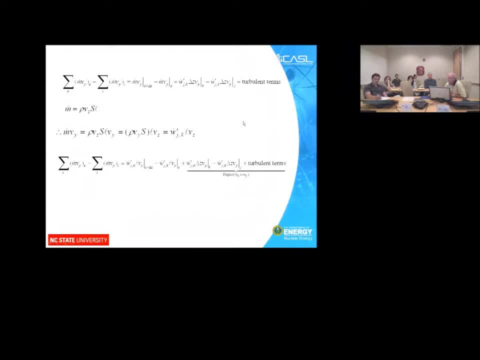 So if you write down all of these equations, then you've got the terms associated with axial flow that transports. so lateral velocity, okay, So velocity moving axially that moves from subchannel j to subchannel k, if you will. But if you've got some axial velocity, 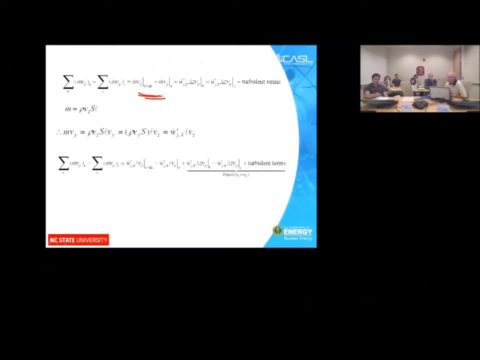 that will transport some momentum in the y direction. you've got lateral crossflows, which also transport then lateral momentum, y, And then you've got turbulent mixing terms. Now, the reason I don't go into a lot of detail about this is because all of those things is thrown away. 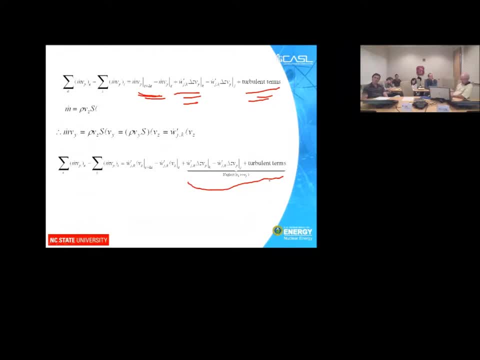 Okay, It is assumed- again- we mentioned this earlier in the assumptions for these models- that these lateral crossflows are very low, very small compared to the axial terms. So in these terms you would have a vy squared term. essentially, 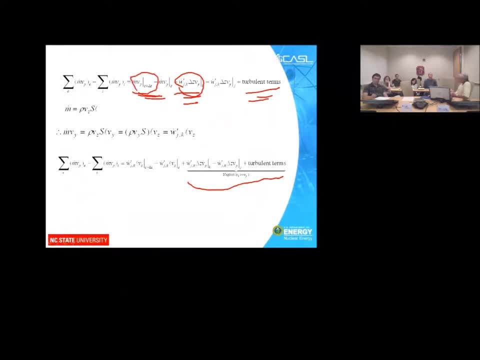 In these terms, you're gonna have a vz vy, And so the assumption is that that vz vy is much, much greater than the vy vy term, And so you just ignore it, And any turbulent mixing terms are also- are also summarily dismissed. 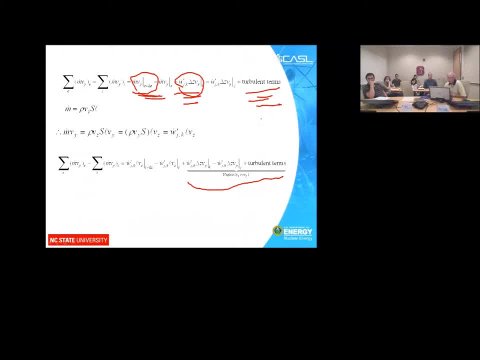 Okay, So they're not even in the model. Okay, And that simplifies the equation significantly. All right, And so now the lateral momentum balance is, in terms of lateral crossflow terms, The forces that we have that act in the y direction. 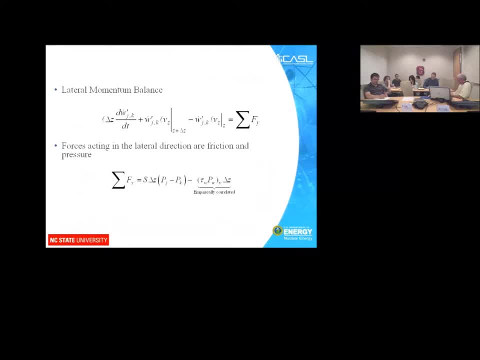 again, assuming that we, that our bundles, are oriented vertically and not horizontally, there is no buoyancy or gravitational term in the lateral direction. So all you have are the pressure driven, the pressure difference, okay, which gives you the lateral flow. 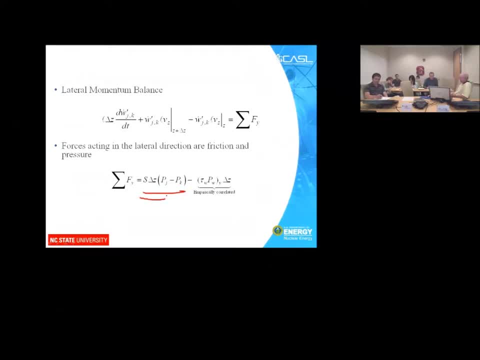 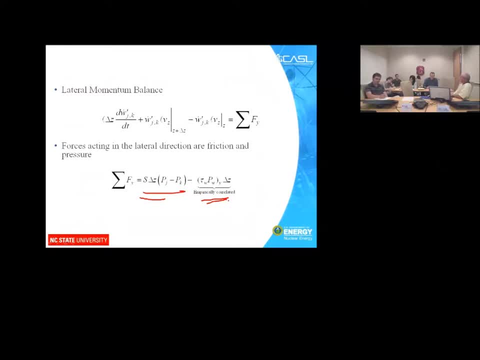 The resistance to that flow across that gap dude, That's called the viscous forces wall drag. Now this is again empirically correlated. Some codes do not give you the option of they'll model this with a loss coefficient. 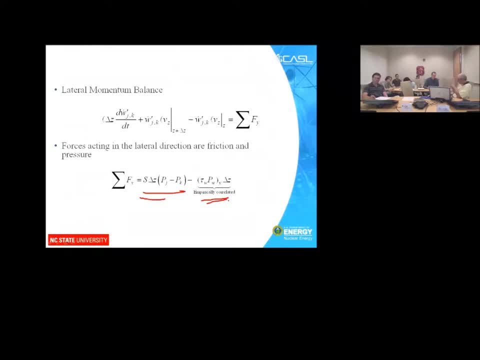 And they'll just fix it in the code: K equals .5. And you have, and it's not an input parameter Now in Cobra TF, is it fixed like that also? That's Yeah, so you don't even have access to it. 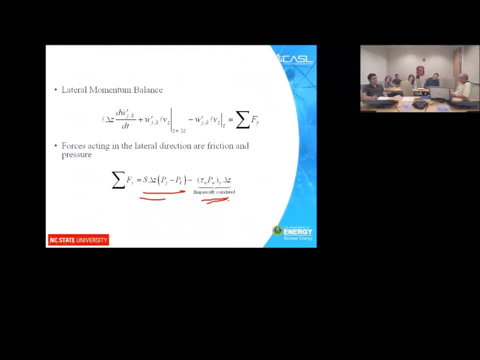 There's not even a correlation for it. It's k equals .5, and that's input, and that's it okay. so, and it would go as this K value the loss coefficient times the lateral velocity squared. so again, most codes, you don't, you don't have. 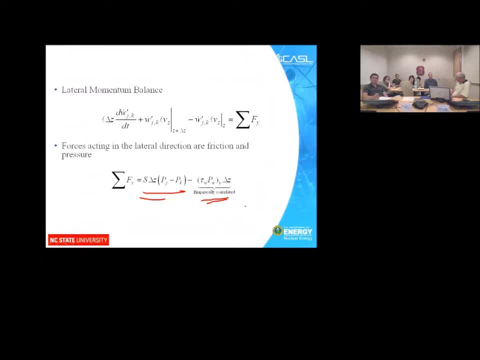 access to that game change. that's fixed in the code. okay, so that would give you then your spatially- you're actually discretized- lateral momentum equation. so this would be applied at every spatial node also where you have options or potential options or adjusting parameters would only be in that term. 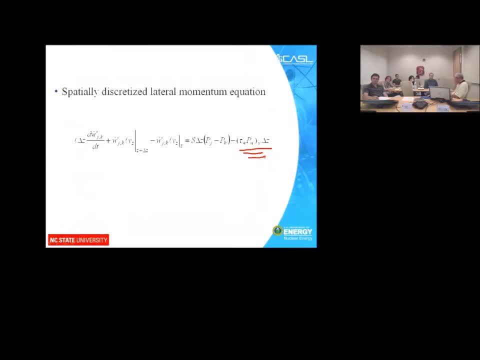 there and it's not available through the input. so in terms of encoder TF, anyway, right now, the only thing that you have access to through the input is going to be the loss coefficients associated with the axial momentum. that's it, the current infrastructure. no, we've also got that chin correlation. well, you don't have any. 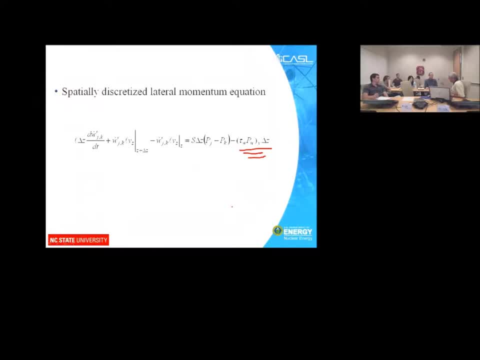 act up- you don't, but it's not physical- or if the correlation was not developed for the pressure and flow regimes that we're currently applying for. so there, people are aware of this, what we've made it aware to them, and it is likely going for, it's going to have to be changed at some point, and when they do so, they may. 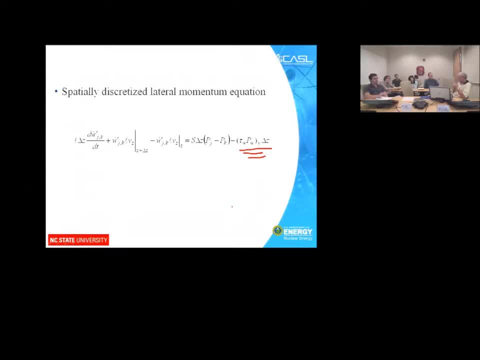 provide options, but it's not going to be short-term, you're not going to have it quick, its not valid. okay, yeah, it was developed for low pressure, high quality. okay, where you have a essentially Angular flow, if that means anything. okay, Where we're looking at is high pressure, low quality, high sub-cooling. 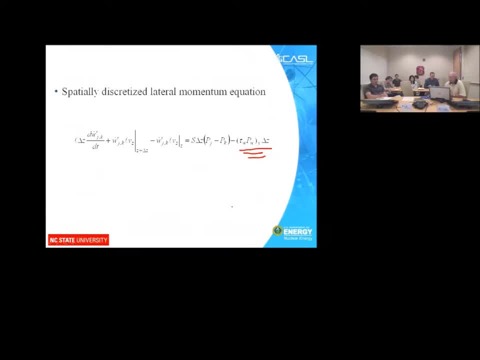 completely different range of parameters. okay, So the change, but it is what's in there and there are no. you don't have any. there's no access to it other than to go into the code itself. physically, You can't. there's no parameters to choose. 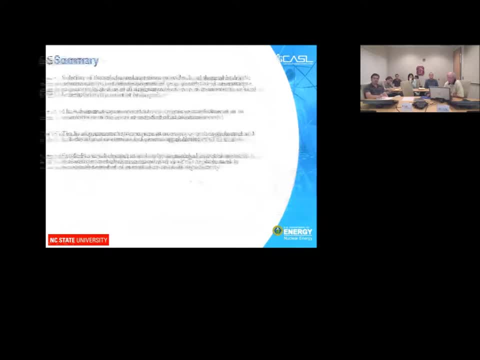 All right, Okay, so let me summarize: This is the last thing, and then we can ask as many questions and discuss this as much as you want to. Okay, so, in summary, and again, whether you're applying this, whether you're looking at COBRA VIPER, the various versions of COBRA VIPER, 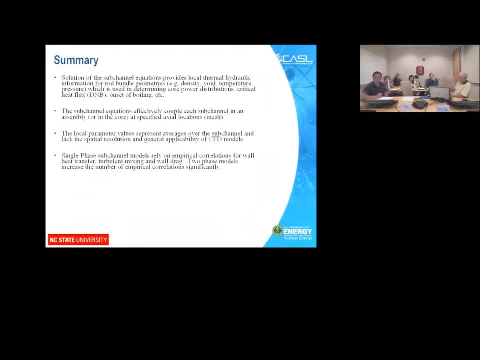 all of the sub-channel codes out there. they're all pretty much based on this same modeling approach. You're going to see slightly different equations, but if you were to go right now and look at any sub-channel manual, you'd be able to look at it and see equations that are very, very similar. 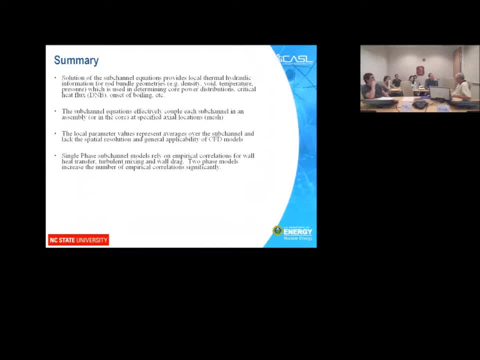 to what I've just written there. okay, No, Relap5 is not. Relap5 is a one-dimensional systems code. okay, so it is not a sub-channel code. What many people do is couple Relap to a sub-channel code. 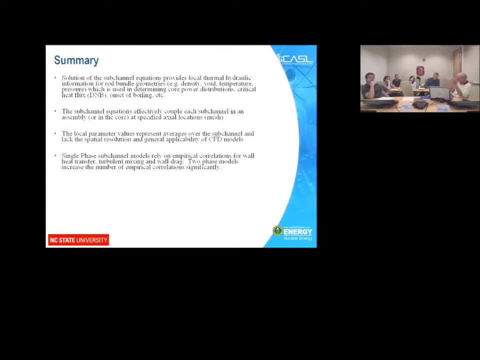 to get higher fidelity in where you have three-dimensional flows inside the core and where that may be important, Then they'll use Relap to provide the inlet and outlet boundary conditions and then COBRA to do the three-dimensional modeling. Look, I am not familiar with that one. 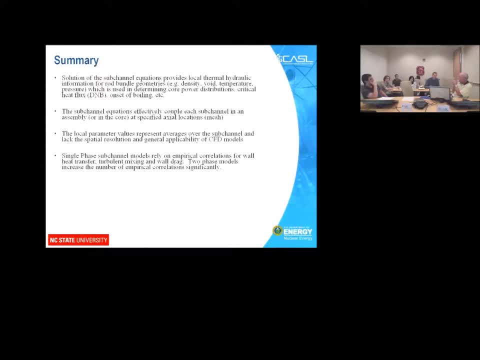 Maybe someone else who's listening in knows It's two things, but I don't know the. Yeah, I don't know. I'd say the sub-channel codes that I'm aware of right now, COBRA and VIPER, are short. 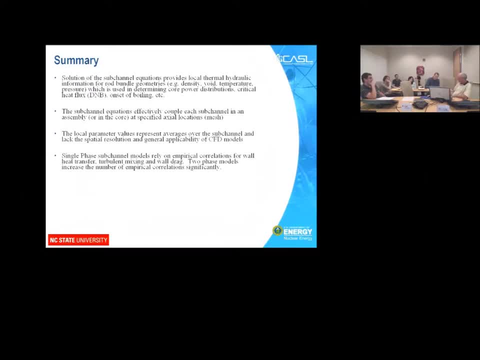 The industry. Yeah, I don't know The industry standards that you'll find. There may be other ones out there. GD may have its own version, but COBRA and VIPER are these sort of standards. Westinghouse, for example, uses a VIPER version. 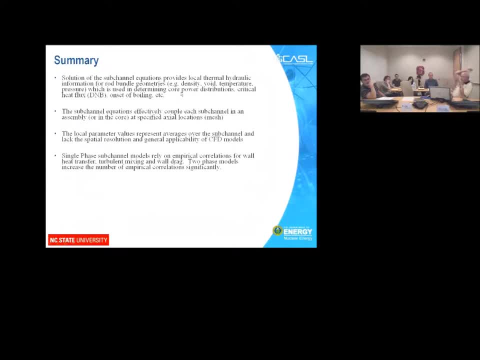 Okay, Okay. So the sub-channel equations give you local thermal hydraulic information, a lot of them. By local I mean it is sub-channel area average. so in the lateral direction the resolution is on a sub-channel basis. Axially you can discretize it in whatever, however many nodes you want. but again, 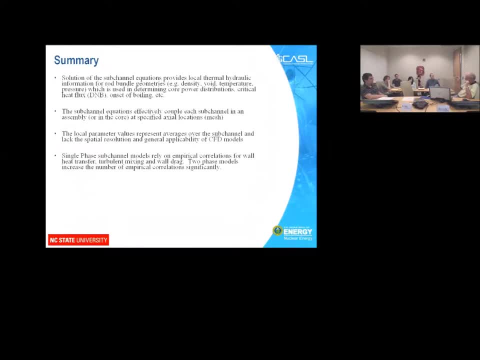 if you're going to be putting in things such as spacer grids and so on that have a two-inch maybe width and you're going to model the pressure drop across that with a point discontinuity, then going to very fine mesh in a sub-channel code in the vicinity of a spacer grid. 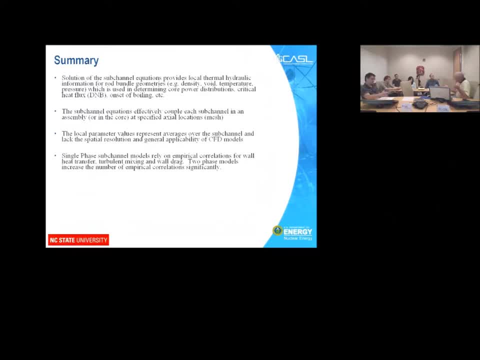 one can question whether or not you're modeling that consistent with the physics. Okay, Now, One of the things that could be done, for example with CFD codes, is all of these empirical correlations such as loss coefficients. the heat transfer coefficient is not modified generally in the vicinity of spacer grids. 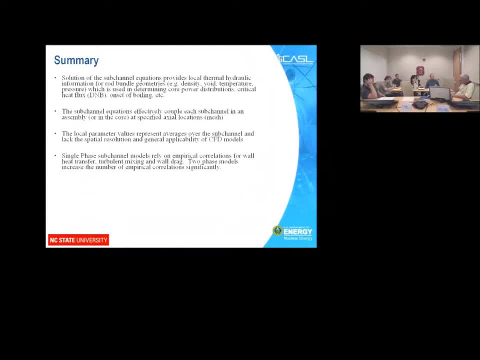 even though it should be Now in some codes they do have the option to modify the heat transfer coefficient some amount in the vicinity of a spacer grid, but it's essentially the exact same correlation That was developed for open rod bundles, applied even in the vicinity of the spacer grid. 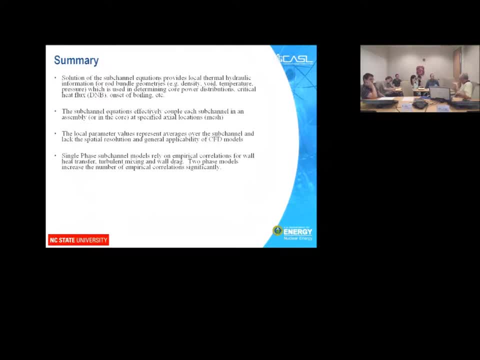 So that obviously is an area where, if you had access to the code, you could modify and look at: okay, what should it be, What should the correlation be in that range, Okay. But if it provides local thermohydraulic information- the rod bundle geometries- again, that's key. 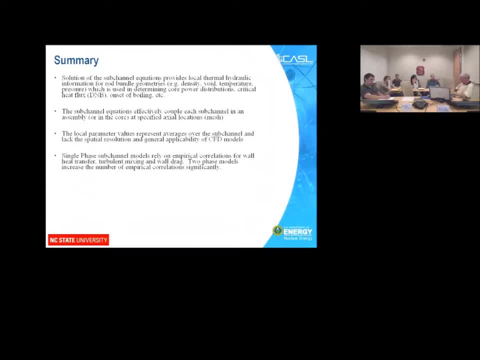 It cannot be used in big open volumes that don't have bundles in them. Okay, It doesn't, Because everything assumes it flows between these gaps and all the equations are developed that way. So it gives you density, void, temperature, pressure, so on, which would be used in calculating core power distribution. 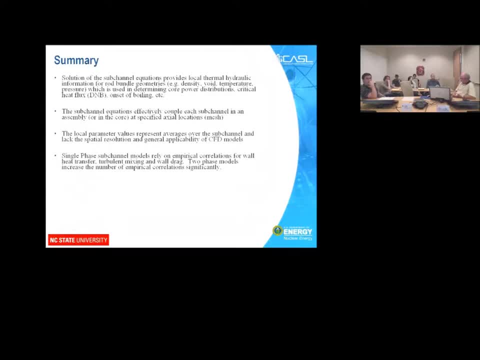 So this information would be fed directly to people who do radiation transport calculations, because they need densities, they need voids. Okay, It gives you temperature, it gives you pressure. If you're doing DMV calculations or critical heat flux calculations, it gives you the local enthalpy pressure. 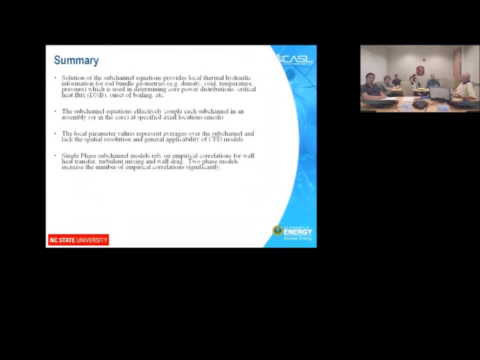 Okay. It gives you the local enthalpy pressure flows that you need for doing that. These calculators, these codes, can tell you at what point you have the onset of boiling. If your heat transfer coefficient is wrong, then you're going to predict the wrong place for boiling. 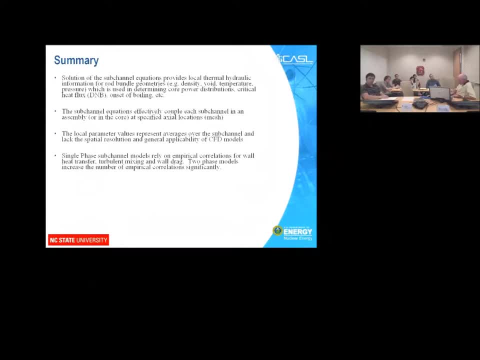 Because most correlations or predictions for the onset of boiling are based on some critical wall superheat, which means that you have to get the wall temperature right And if the wall temperature is wrong, you're going to get temperature wrong. Okay, Okay. 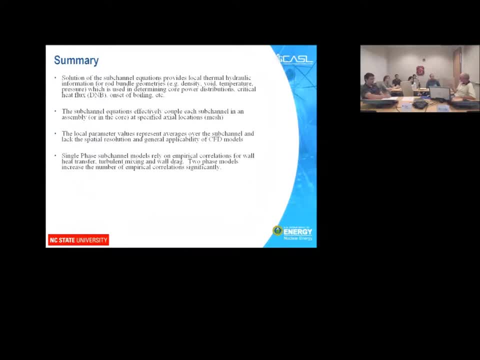 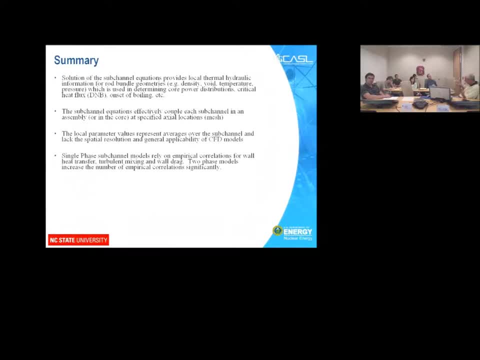 At each axial location. Yes, Yes, Yes, Yes, Yes, Yes, Yes. Now that resolution 50,000 lateral by some number of axioms in CFD talk may not be that many, But that would be a large subchannel calculation. 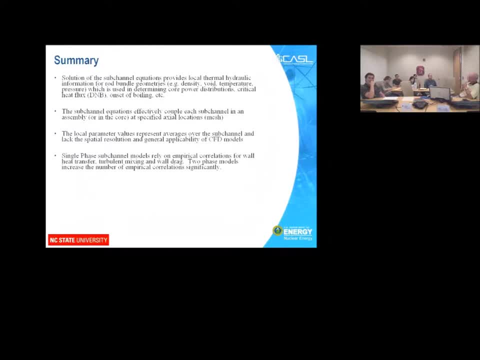 And, as a consequence, many times they do just assemblies or quarter cores or whatever when they run these. So again, the local parameter values that you get are averages over the subchannel, So you don't get any spatial resolution within the subchannel. 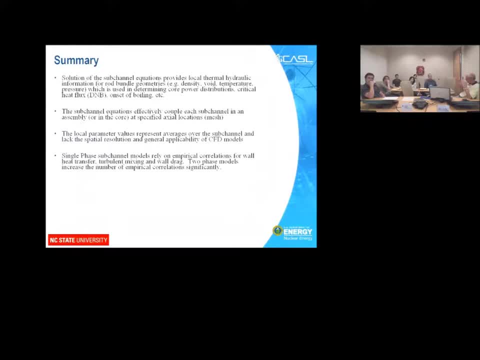 And so, again, it lacks the spatial resolution and the general applicability that you get from CFD-type calculations, The single-phase subchannel models. we've talked to rely on empirical correlations and we talked about where your wall heat transfer channel mixing wall drag. 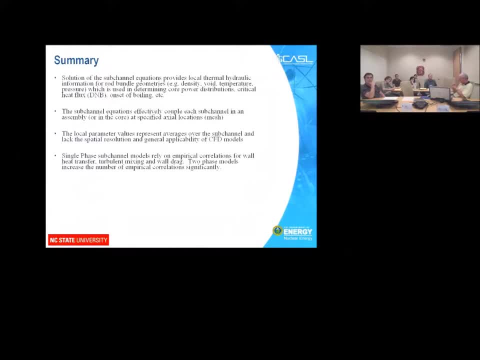 When you go to two-phase, then the number of empirical correlations that are involved explode, Because you've got not only the same sort of correlations for each phase that you have in single-phase, but you also have all of the interfacial interaction terms that occur. 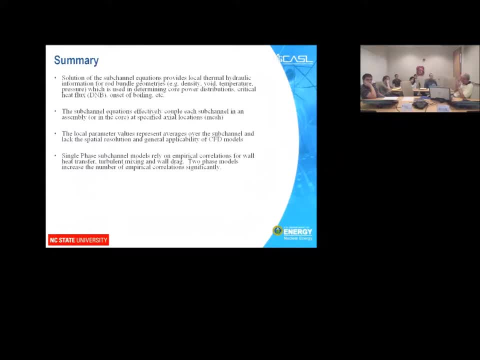 Now these again in COVID-TF are hardwired. You have no opportunity to choose them or to modify them. They're hardwired. So all I've mentioned here is that the two-phase models increase the number of empirical correlations. 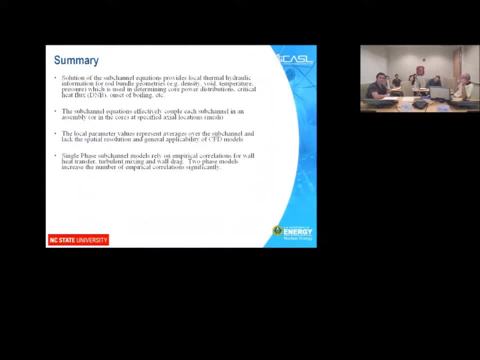 significantly, And anyone who has looked at two-phase models, whether it's subchannel 1-Z, systems code, do not know that there's a fairly large range of data spread for the correlations that are in these things, even though we understand them fairly well. 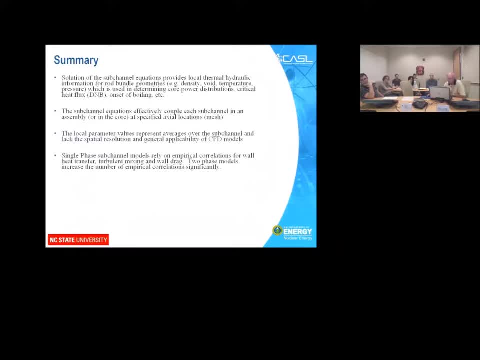 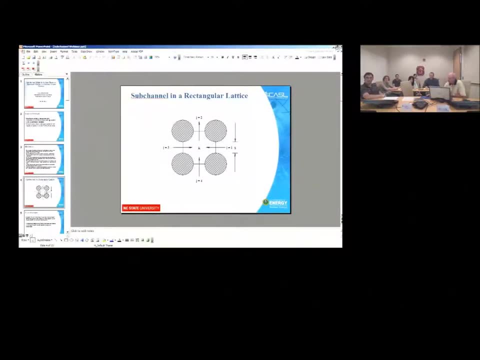 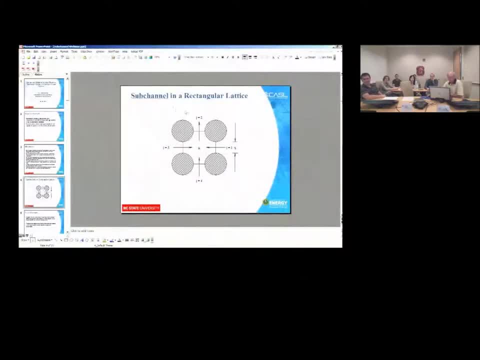 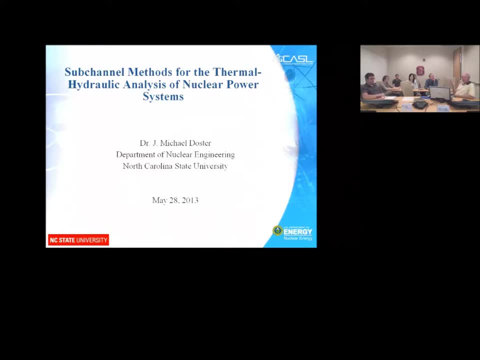 The purpose of this was again to provide sort of a To give you some idea of what the sub-channel codes do. No, no, That was great, Thank you. All right. And to give you some area of if you're doing chemistry and you need local conditions, they're going to couple two decide. 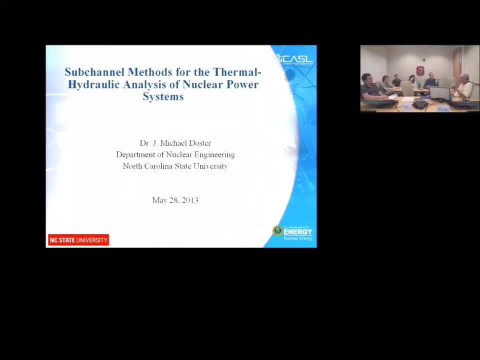 everything together. Yeah, Everything that we're doing in CASEL is going to be coupled to these sort of calculations at some level or another. So the neutronics, the chemistry, the BUQ, all of this, maybe the only thing that's not. 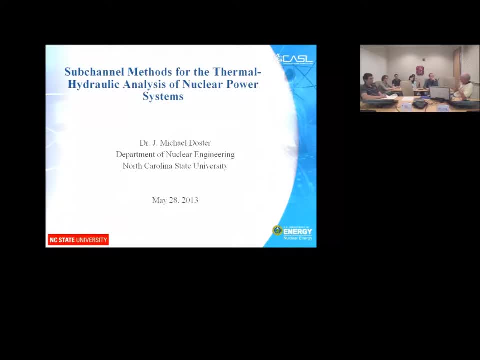 is the fluid structure and even that might have some couple. I'm not sure, But there is. there are opportunities here for doing data simulation or doing parameter characterization, to do sensitivity and certainty. When the neutronics people are calculating power distributions, they're going to be connected.